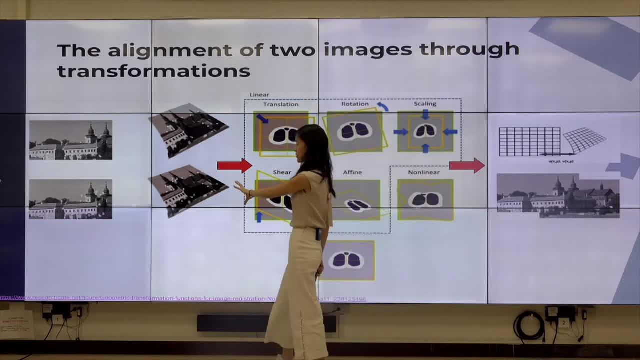 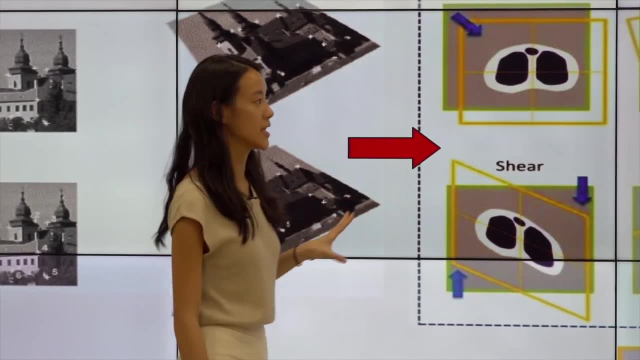 seeing is that we have that image at the beginning. So when it's disoriented, as you can see in this case- so originally you should be looking like that, But when it's disoriented- what registration does is that it goes through a set of these processes so that this image can go. 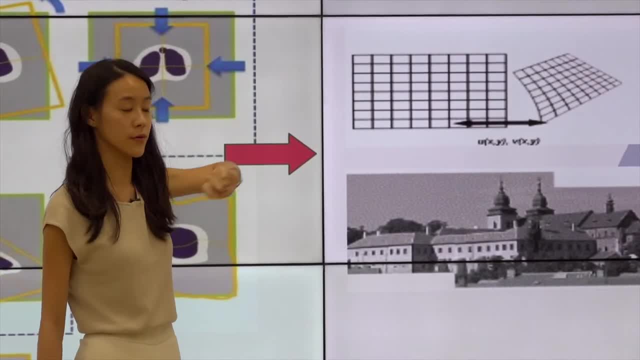 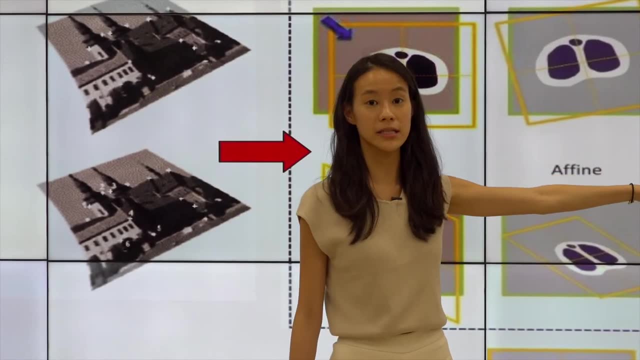 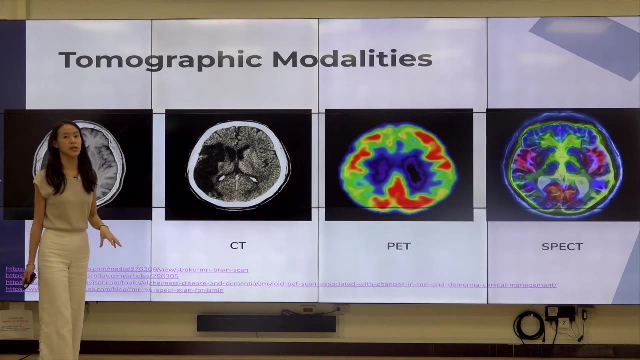 from that disoriented image to something that is more flat and more readable so that we're able to get a better sense of what image we're actually looking at. So we're not able to identify this last part from these two images, And so, with registration, a lot of times it includes different modalities, So a lot of the times we 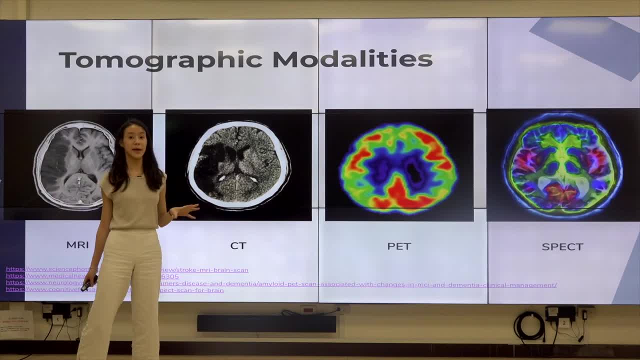 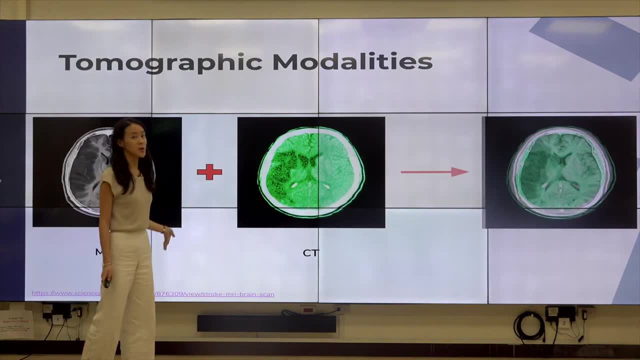 would use MRI scans, CT scans, PET scans and SPECT scans, But for the sake of our purposes today, we're only going to be focusing on MR and CT scans. So to combine all this knowledge that we talked about before by using MRI and CT scan in order to register these two images together. 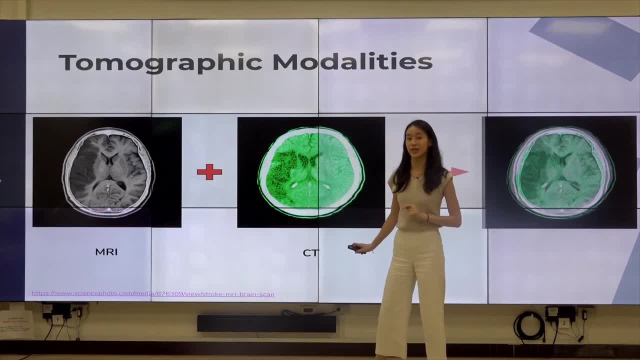 this is exactly what it looks like. So originally the CT scan was not in green. I changed up the color a little bit so that you guys can get a better sense of what I'm talking about. So what happens with registration is that we have these two different images. 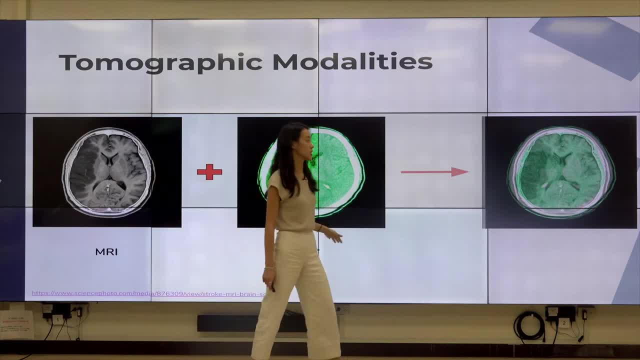 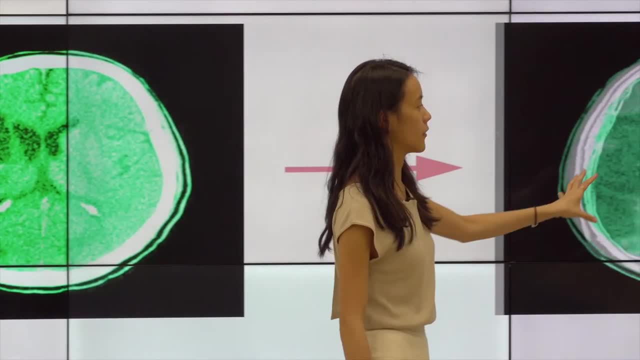 at the beginning and our output after registration should be the compilation or having these two images overlap, so that we're able to get a better sense of what we're looking at when we're comparing these two different images. So it should align in some sort of way. so 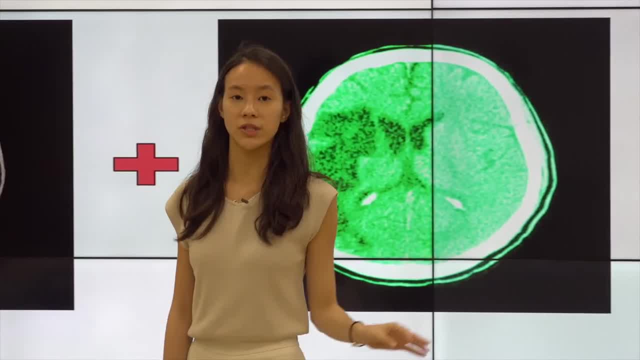 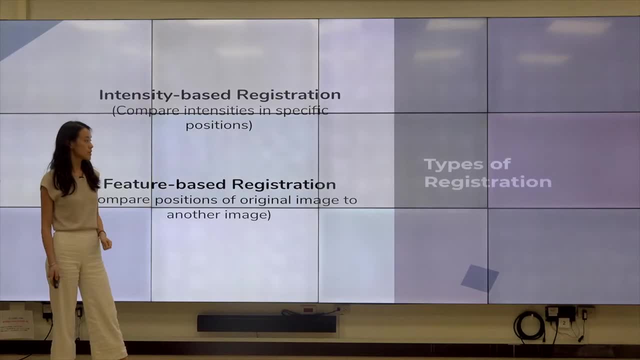 that we're able to be like, hey, potentially this tumor is in this section, which is the same section as the other image, or maybe even off in the other image. So there are two different types of registration that I would like to share with you. The very first kind would: 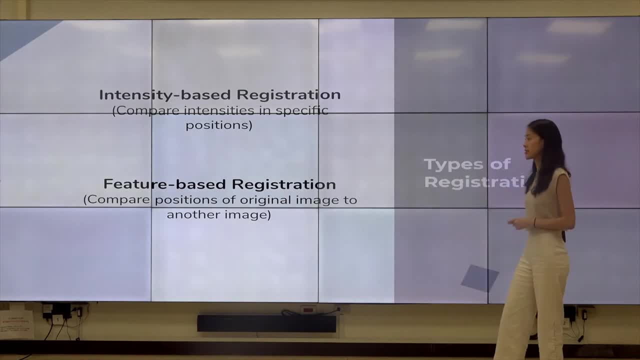 be the intensity-based registration, and the second kind is the feature-based registration. So one thing to note about the intensity-based is that it is comparing the intensities in specific positions. So the way that I would like to see it is that for each of the pixels, 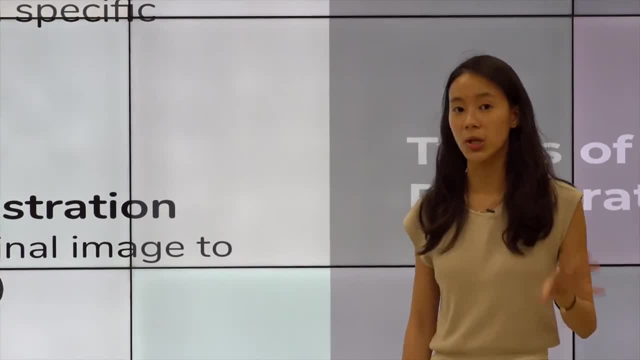 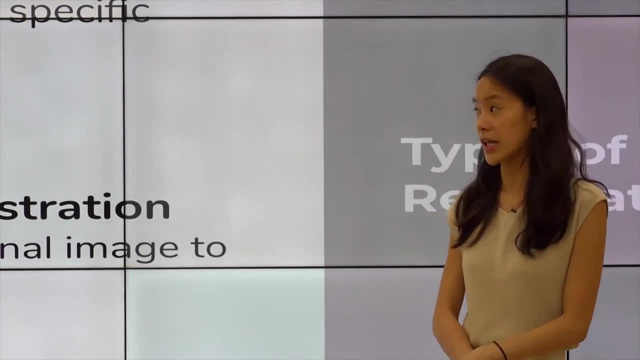 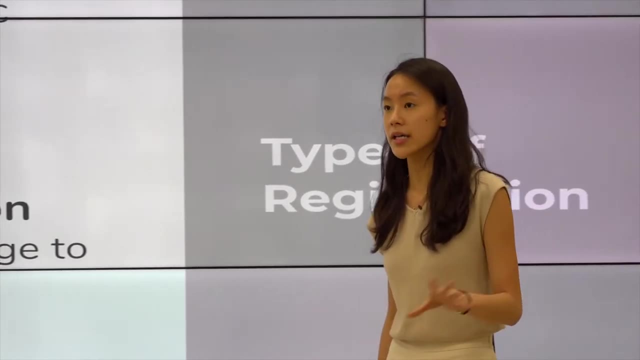 that we're looking at. intensity-based registration is actually looking at these individual pixels or these individual positions, and compares the intensities in order to be able to register the images together. The feature-based registration actually compares the positions of the original image to the other image. So I would like 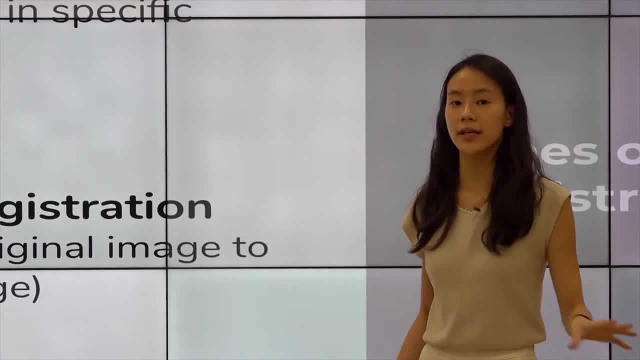 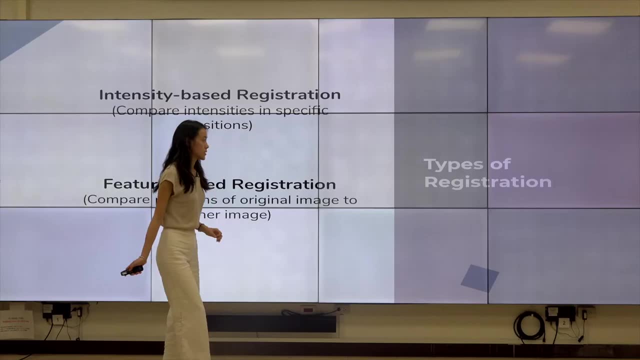 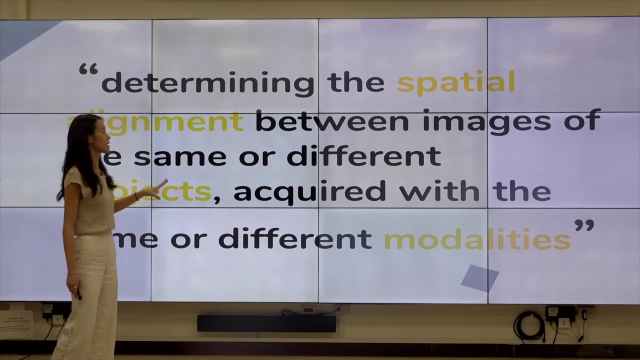 to view this as a more overall. So what ends up happening is that we're viewing the entire image during registration, as opposed to a single pixel, And so one thing to note is that, as a summary of what registration is, it is determining the spatial alignment between images of the same or different subjects acquired. 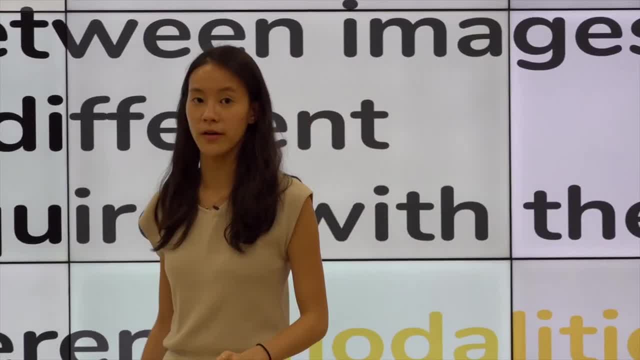 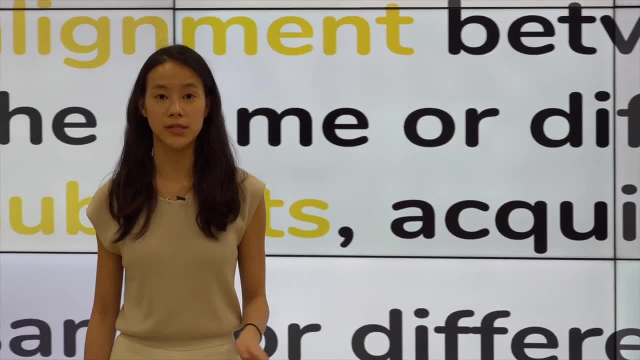 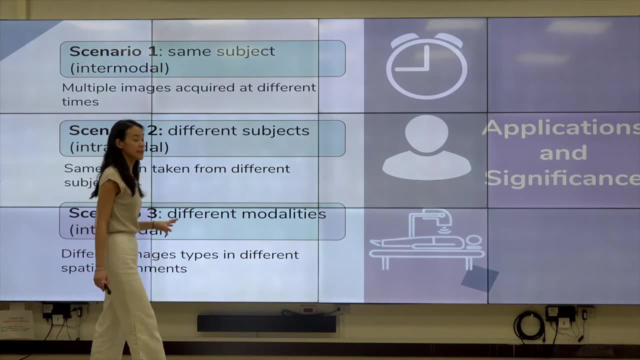 with the same or different modalities. So that's something that we're going to go into a little bit deeper in the remaining of the lecture- where registration can occur in multiple kind of scenarios and in multiple kind of situations. So, talking about the significance of registration, So the applications and significance, as I stated before, 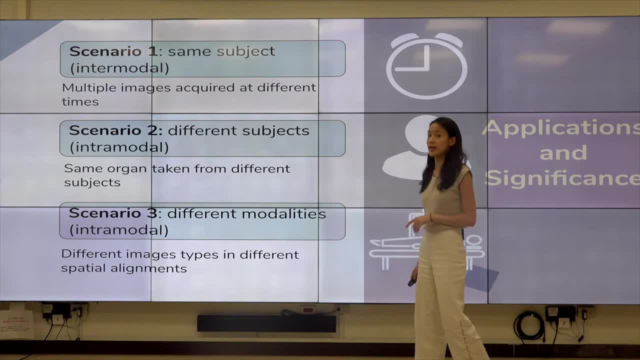 that summary of what registration is can occur in three different kinds of scenarios. So the very first scenario would be the same subject which is considered as intermodal, the, the phrase for that, and basically what happens is that we may have multiple image acquired at different times. 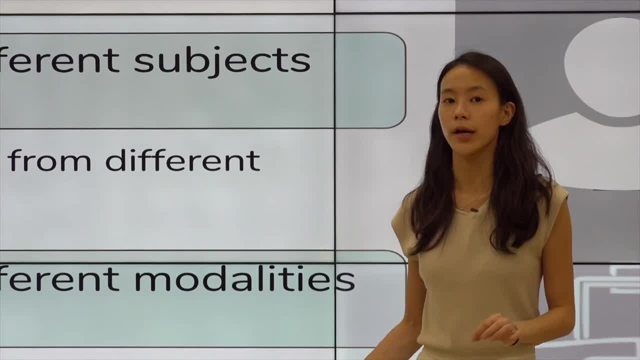 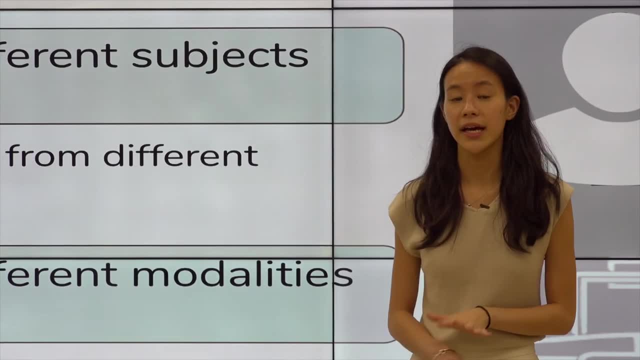 and this may be in the morning or in the afternoon or at night, where we have these different scans that are taken at different times and due to a lot of biological reasons, as I'll explain later, it is very- there may be differences in the images, so it won't be the same if we take it. 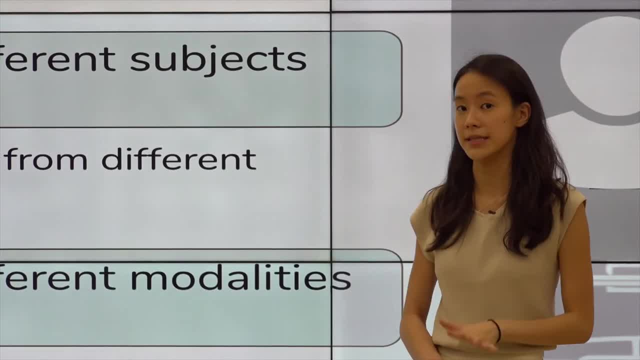 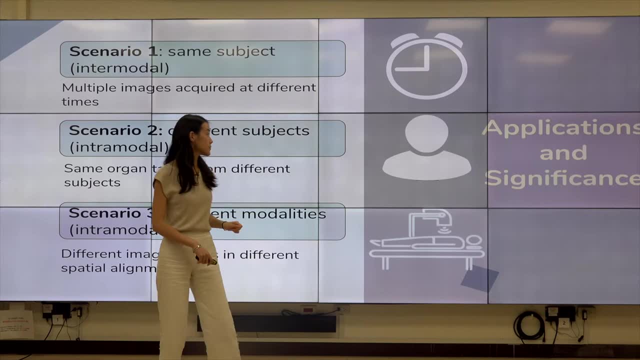 in the morning, in the afternoon and at night, the images would not be the same and because of this, we would potentially need registration for the same subject or the same person. Second scenario would be for different subjects, and this is considered as intramodal, and so for different subjects. it could be potentially a situation where you're 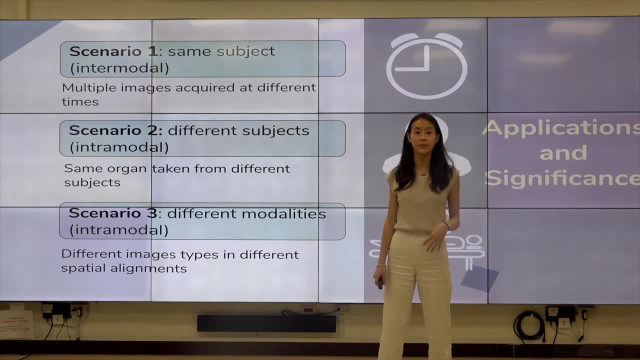 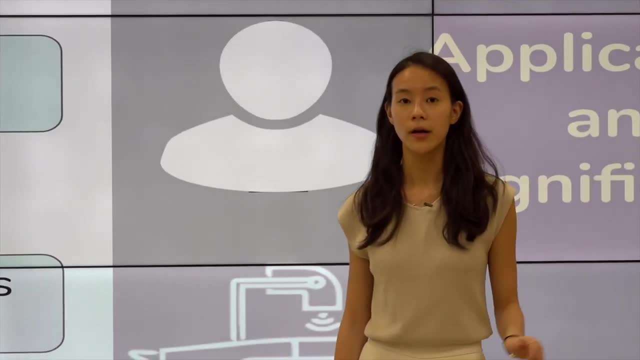 comparing five different kinds of subjects or five different people who have brain tumors. however, they may be in different locations. so if you're looking at the images or you're trying to compare, maybe this tumor has a tendency to grow in a certain area of the brain. what we end up having? 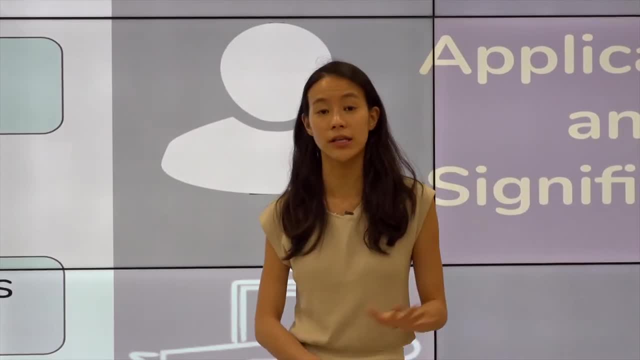 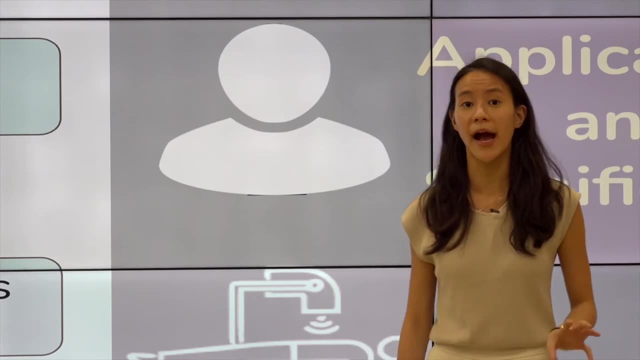 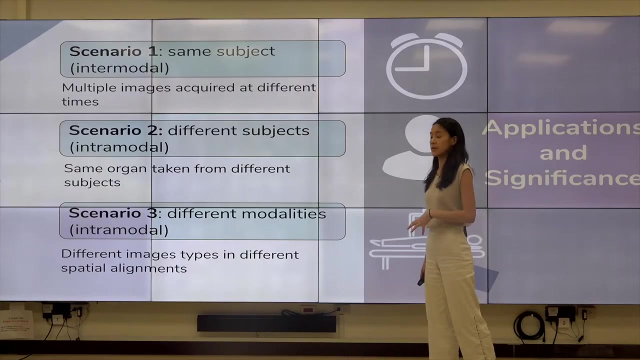 to do is that we can register all these five different subjects together, or the images of all these five different subjects together, in order to identify: hey, maybe there is a specific region where this tumor actually grows. So that's where registration is important in scenario two and so scenario three would be different modalities. 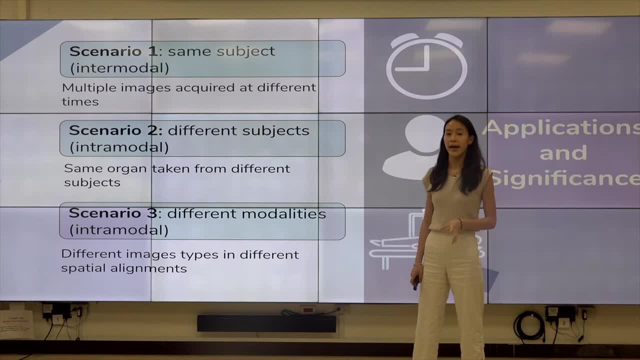 So this would be considered as intramodal as well, and the different modalities were mentioned at the beginning, where there were four different kinds of modalities, and so this may be a situation, or may be significant in a situation, where a patient is being transferred from hospital A to hospital B. 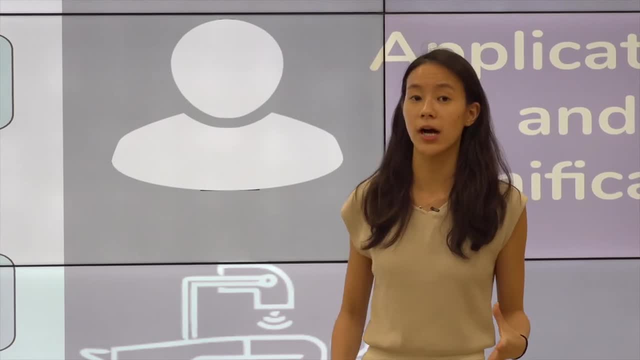 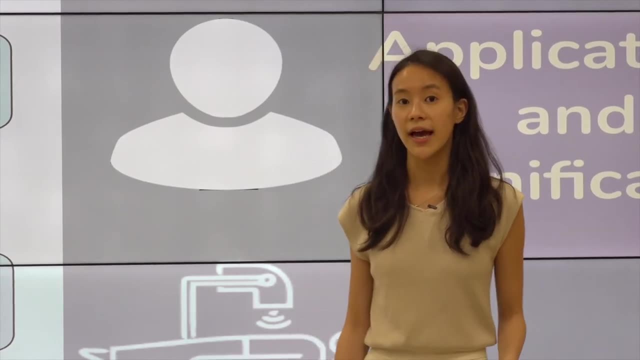 and in this situation, maybe hospital A doesn't have the resources that hospital B has. So, for example, one of them only has MRI scans and the other only has CT, a CT machine, And so in this case, by having the results that they're getting, they're actually going to be able to identify the 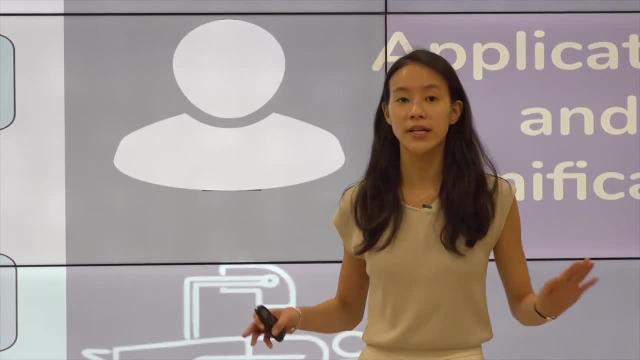 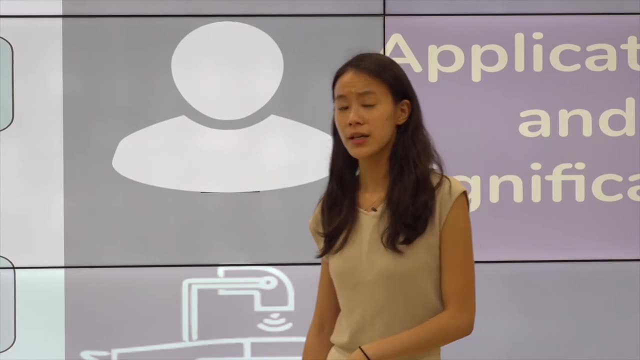 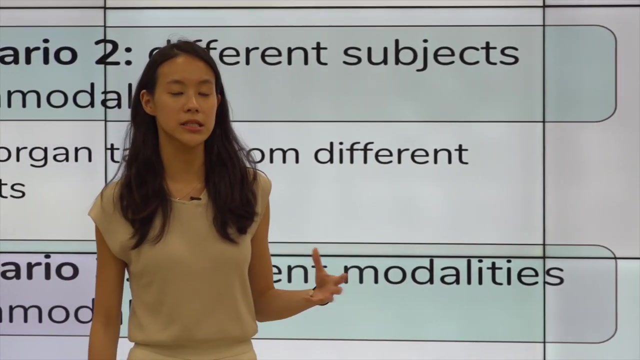 a registration process, we're able to register these two different images together as the patient is getting transferred from hospital A to hospital B, so that the doctors are able to, I guess, in a sense, compare or analyze this patient's, this patient's condition or the situation, maybe the 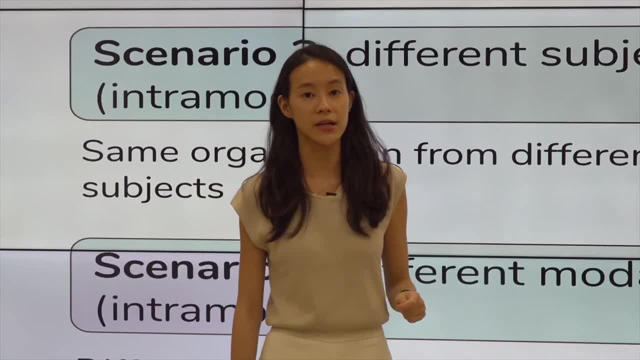 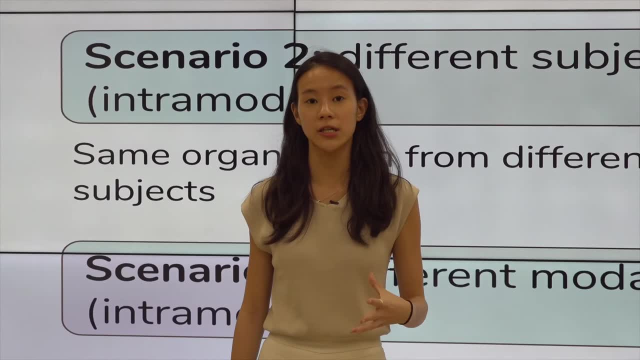 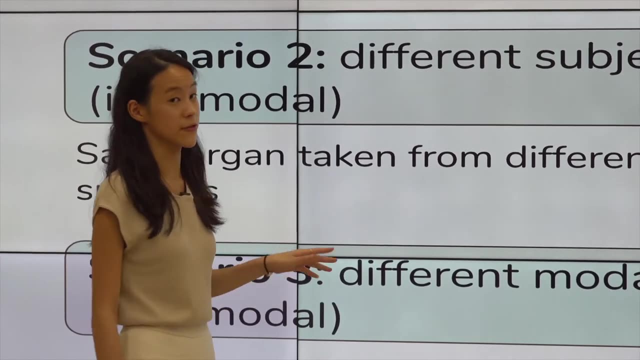 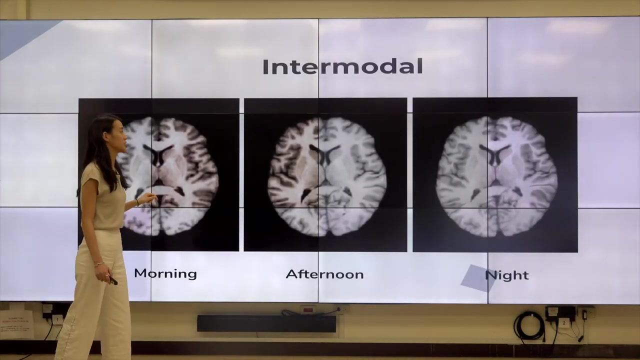 scan was taken three months ahead before, or maybe it was taken six months- and seeing that disease progression is very important for the physician in order to identify tumor types and the progression of treatments or the effectiveness of treatments. so this is where registration may become important when we're talking about different modalities and so an intermodal situation, as I explained. 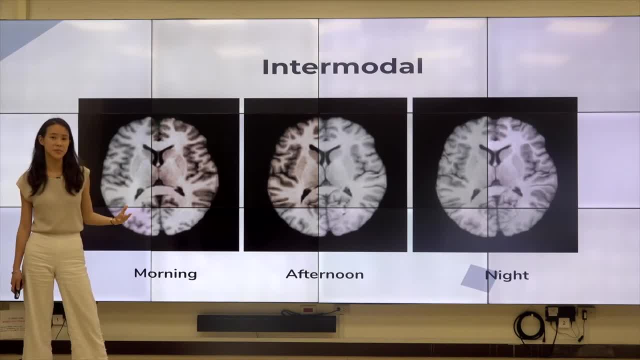 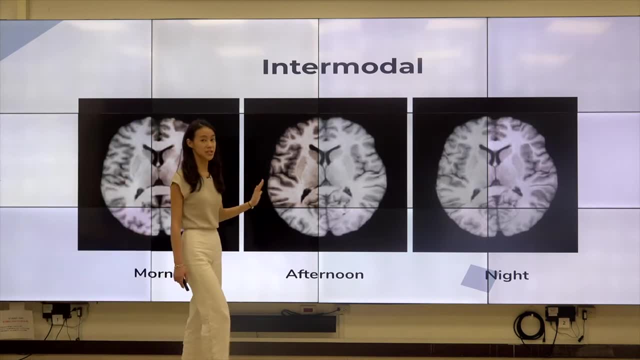 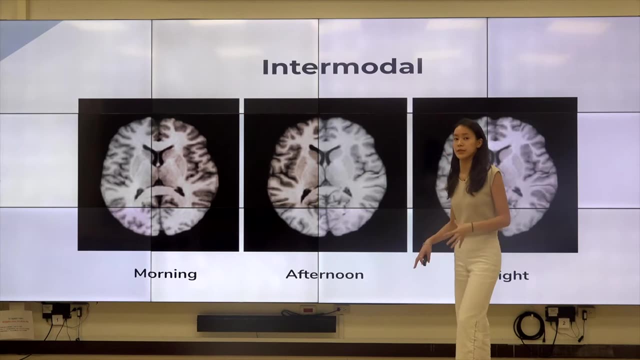 before would be a situation where we have the exact same subject but taken at different times, and so in this situation, as you can see, these are three different images together, taken at different times- morning, afternoon and night- and, as you can see, from the naked eye we can't- there isn't a very obvious difference between all these three of the images. however, 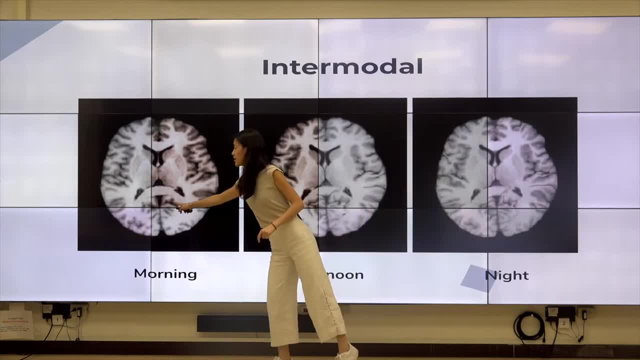 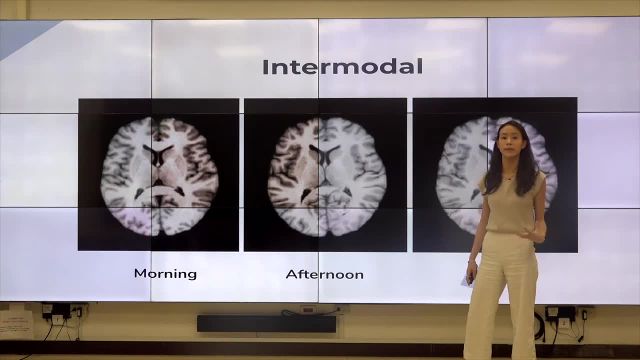 the truth is that there is a difference, as you can see here in this section it is very different from the afternoon section, so that's something that it would be very hard for us as human beings to pick up immediately, but for a computer registering these two images is going to make. 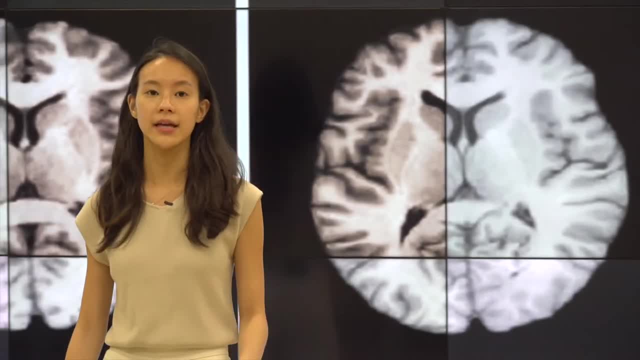 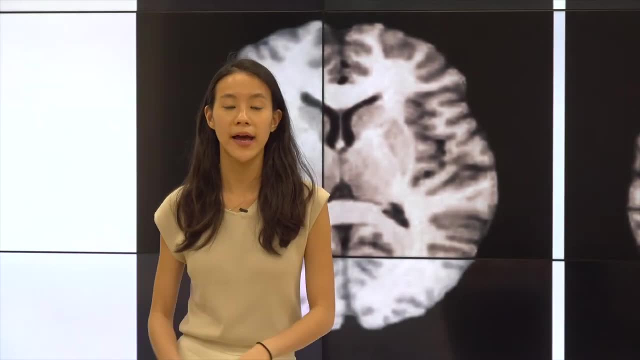 it so much easier when we're overlapping these two things together and being like, hey, there's a difference in this area, and you can think of this as one of those childhood games that we used to play, when we would have multiple, we would have a lot of distractions and it would ask you, for example, 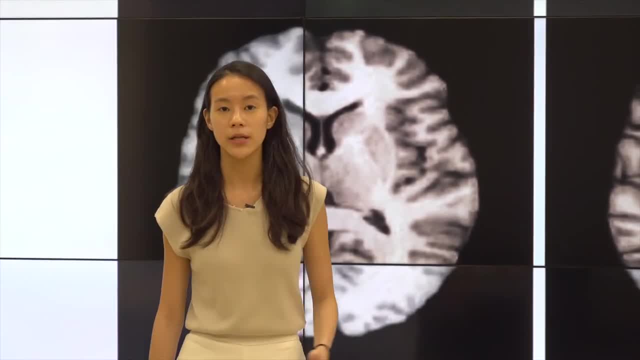 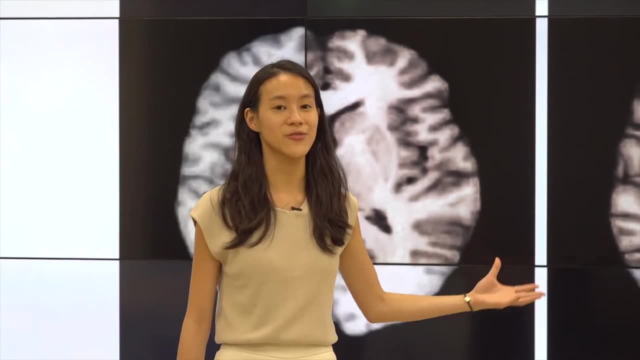 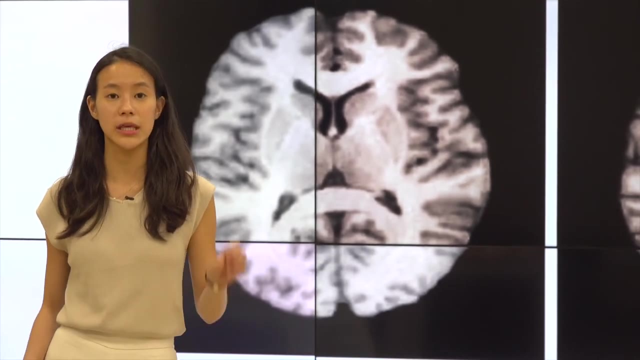 to find a specific character, let's just say Mickey Mouse. let's find the number of Mickey Mouses that you would see in this area and potentially in this situation. registration would be comparing these two images together, where most of the most of the image would be the same between these two different images, but there would be slight differences in certain. 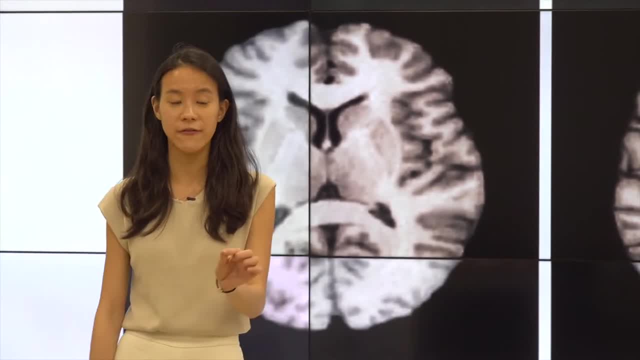 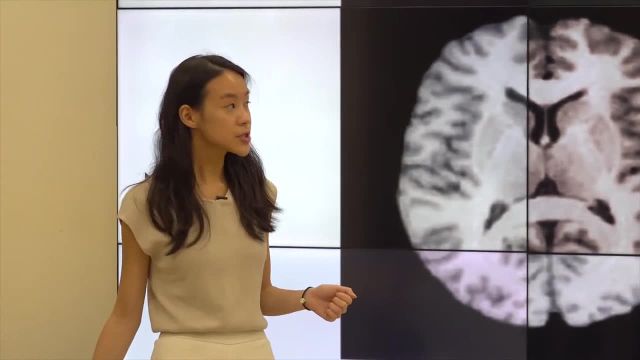 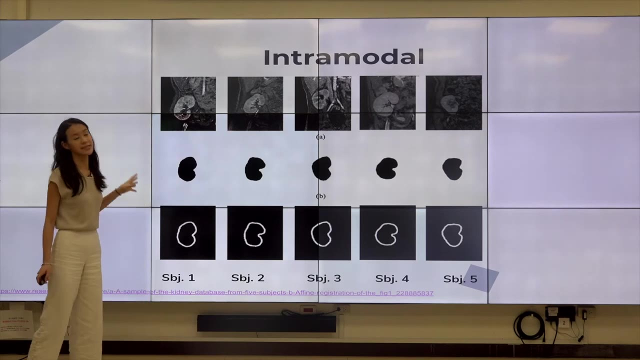 areas, and by registering these two images together, you can identify the differences in the small areas that we're trying to look at. looking at a intramodal situation, we can see in this case, which is between different subjects, and so one thing to note is that this isn't of the brain, this is 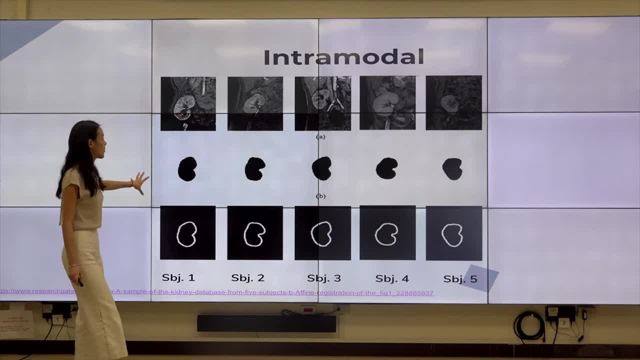 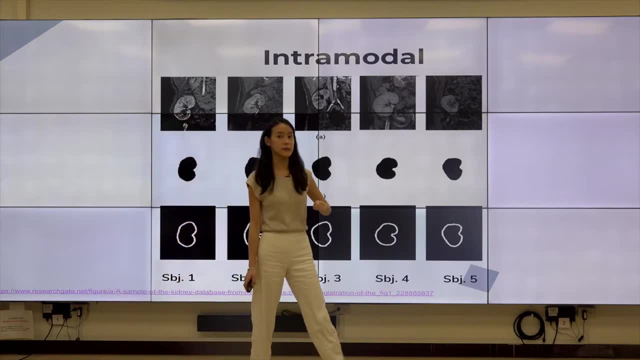 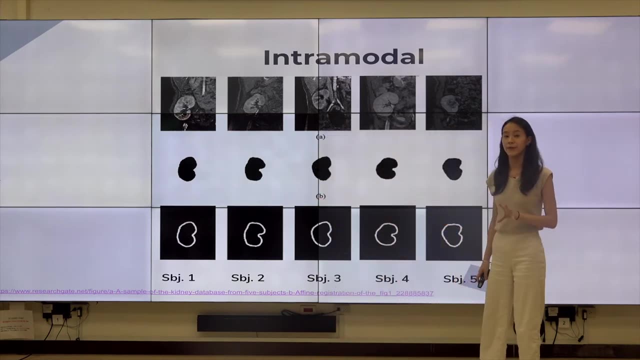 actually of the pancreas, but uh, or the kidney. sorry, but one thing to know about this is the fact that these are five different kinds of patients with the same MRI scan. however, as you can see by these masks, there are very. they're very, very, very different and for a 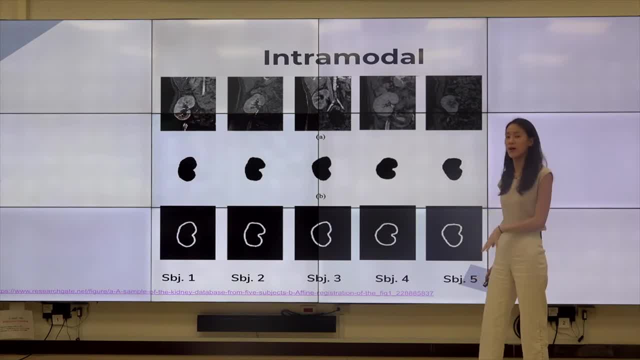 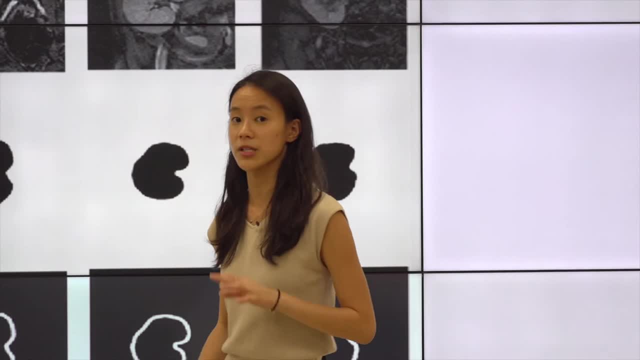 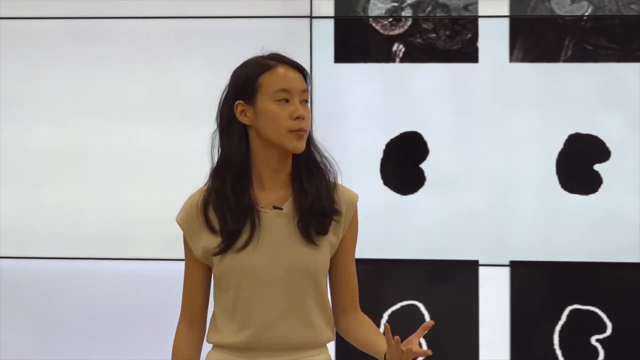 doctor to be able to look at the difference between each of these kidneys would be very hard without registration. so, through scaling, through rotation, through a lot of all these different processes that we're going to talk about later, it would make a physician's life a lot simpler when we're, when they're trying to compare, for example, where the tumor is growing. 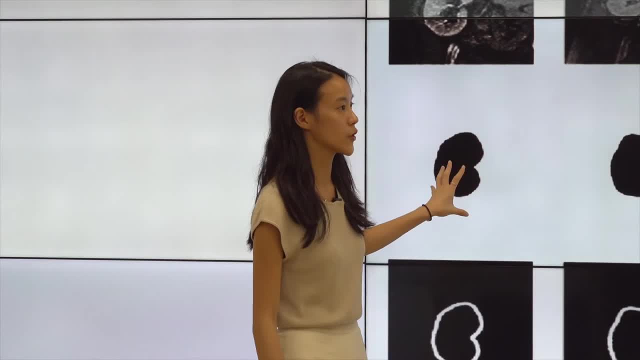 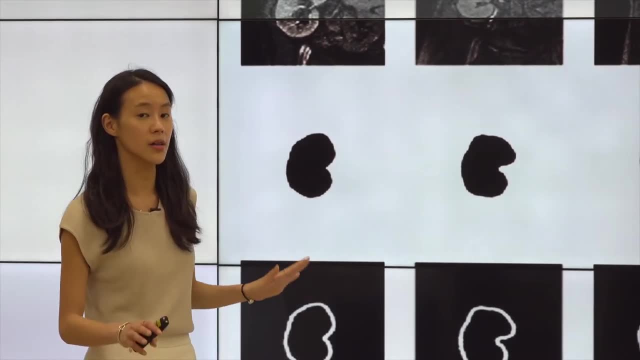 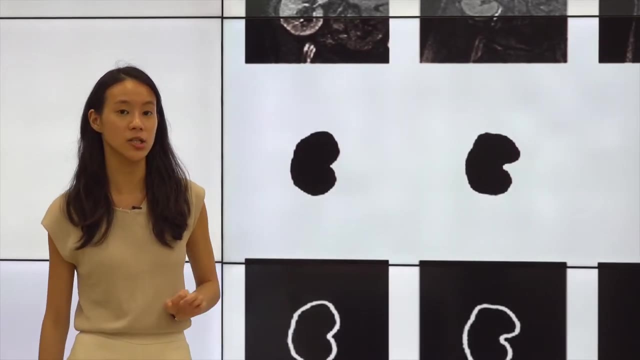 let's just say there's a tumor that was growing here and in order for the doctors to be able to compare this with the remaining of the patients- whether or not that tumor is growing there- would require a lot of registration or a registration process in order to immediately identify how off that tumor is in terms of positioning in each of these patients. 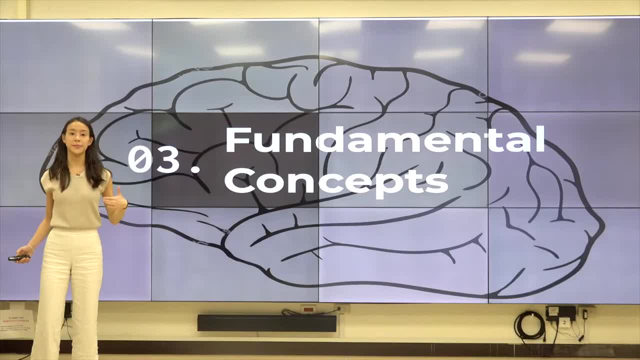 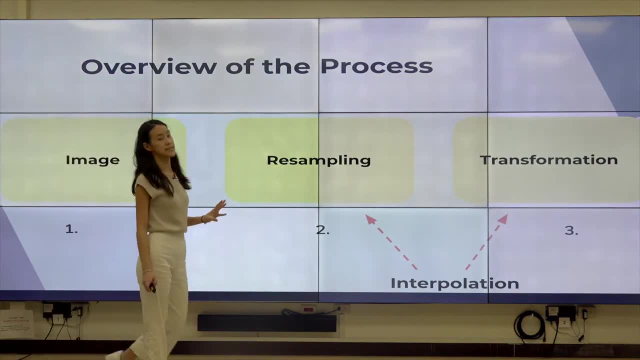 think of it as a more precise measurement. so, going on to the fundamental concepts of registration, so the entire process, as I would like to see it, this is a lot simpler than the segmentation classification that we saw before. in terms of this entire process. there is a image that comes in, so I'm going to be talking about how the computer reads the image, and then 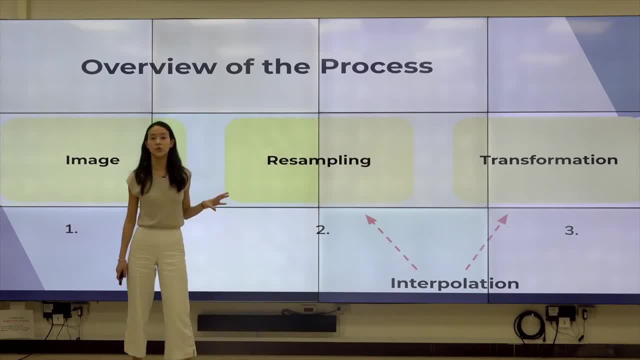 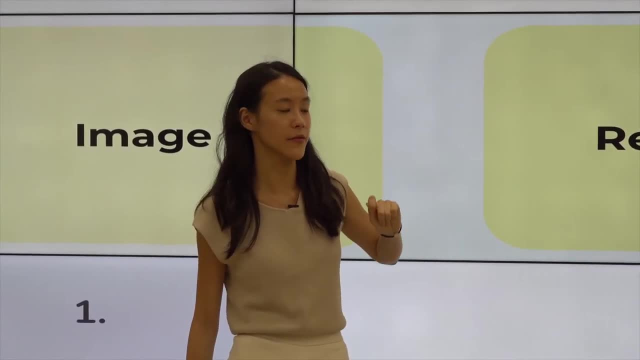 we're going to be talking about the resampling process and then the actual transformation process, which is where registration occurs. so these are the very important steps that are part of registration, and one thing that I'd like to note is that I didn't have interpolation as its own. 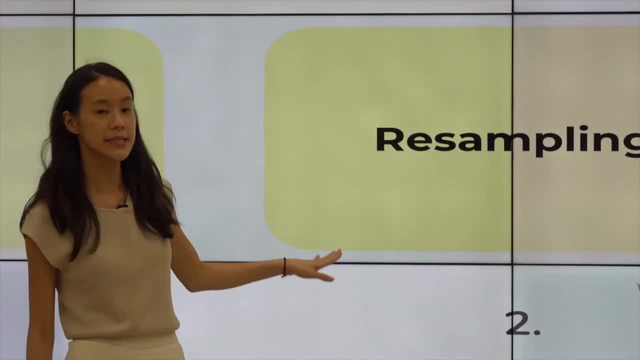 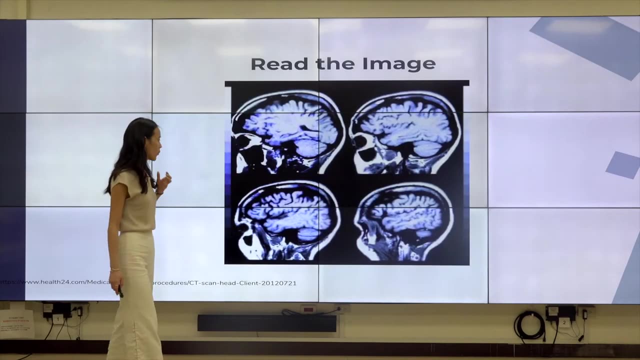 category, because interpolation actually plays a role in both the resampling and the transformation process. so how does the computer read the image? so one thing to note is that, while we're looking at these images, it is very simple, as I explained before, for the human to, for the human eye or 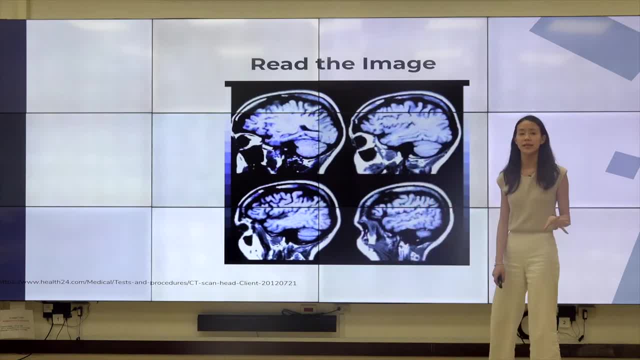 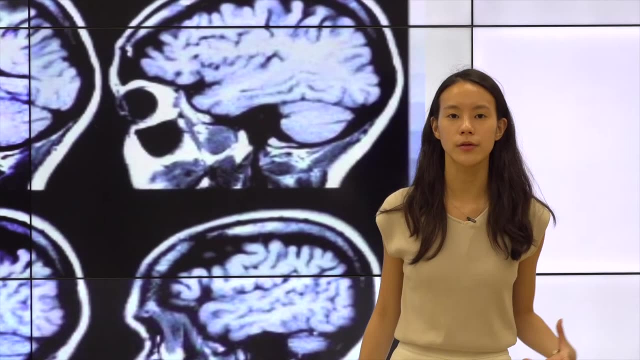 the human brain to see these images and immediately see the features that we have been trained to recognize. so in this case, for example, we would see this as the eye, so or this is the brain and this is the skull, and this as, essentially, the nose. however, for a computer, they don't read the images in this way, as we saw with 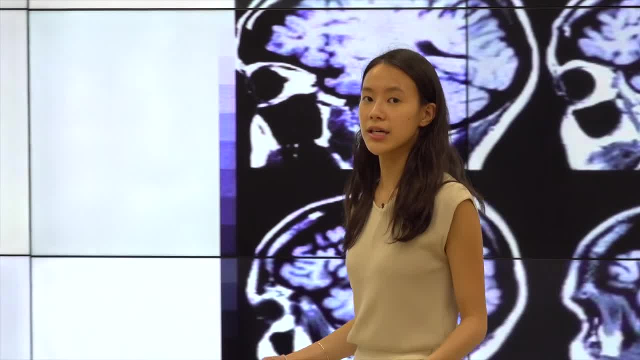 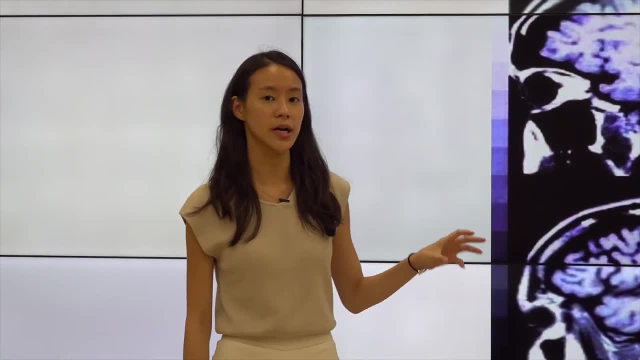 that elephant situation in the classification lecture. a lot of the times the computer reads this and all they see is pixels. all they see is numbers. they're able- they're not able- to register or assign each of these pixel numbers to a feature that we would- we as humans would actually. 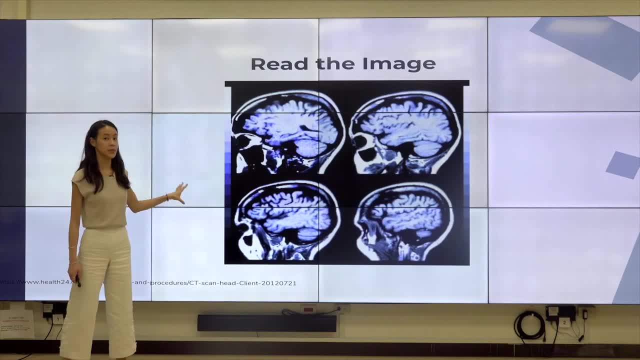 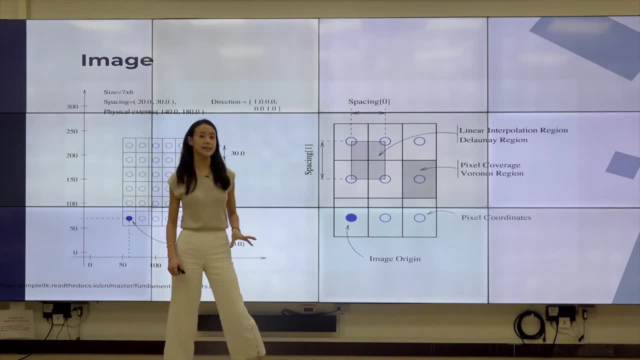 recognize, so reading the image is very different for a computer as it is for human beings. as a result, a lot of the times this is in. this is a diagram that is obtained from sk learn, because this is how they usually read the images, and what ends up happening is that, as we input an image, 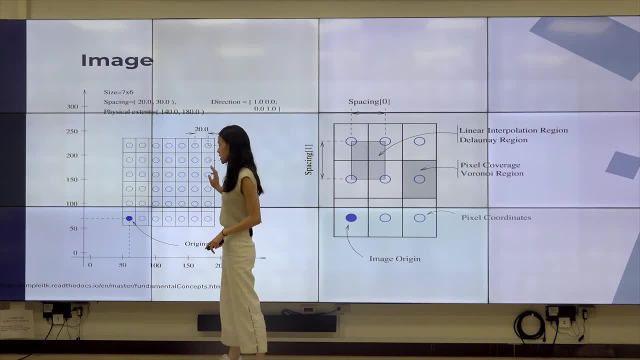 into the algorithm. it assigns that image to different values. so first thing that they would do is to define the origin, and then we would have the pixel width, for example, or pixel height, and that would be noted in terms of the, in terms of the spacing for each of these pixels, and then we would have the direction, so in which? 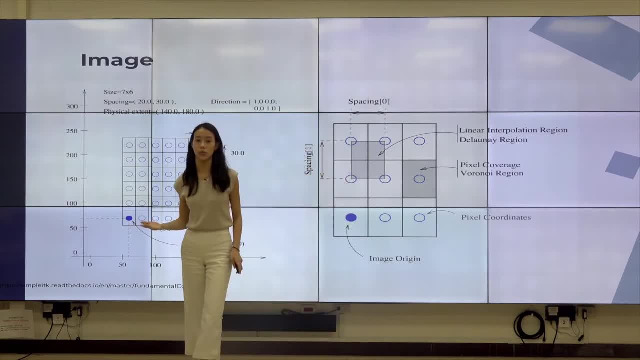 way is the image oriented on the axis that we're looking at, and then going in deeper, in deeper details, what we see is that, as we're talking about, this is spacing one and spacing two, so the height and the length of each of these pixels, and one thing to note is that this: 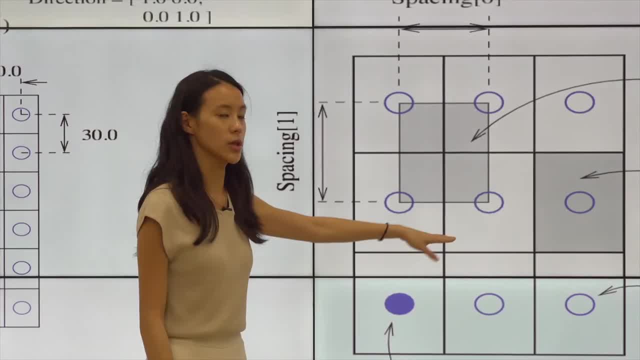 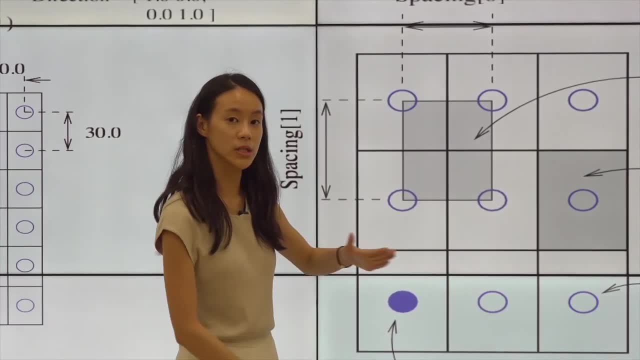 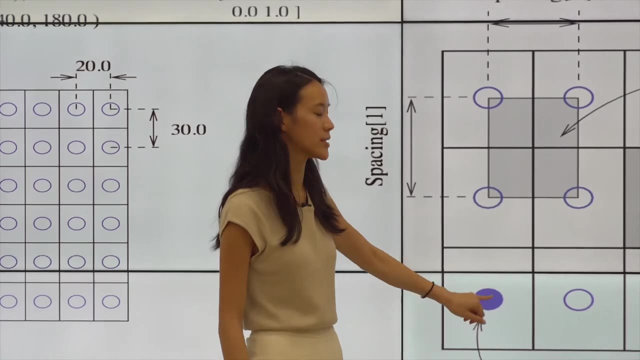 is the image origin. so every single time, a lot of times, when we're looking at diagrams or grids, we tend to note or we tend to see that middle part where the two lines intersect as a point. however, when we're reading images, or when the computer is reading images, what it tends to do is that middle. 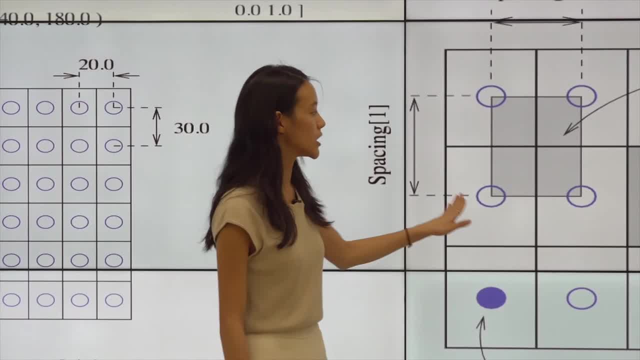 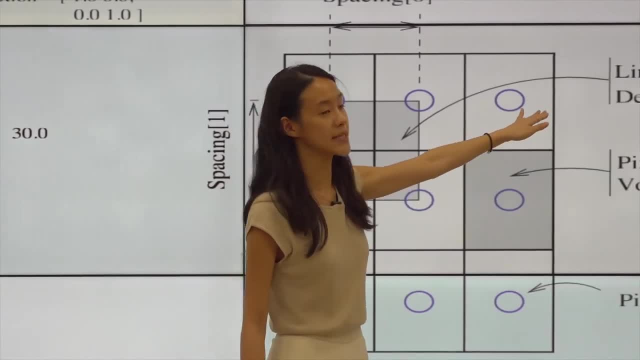 point of the spacing grid that we have defined. so each of these middle points is what we're going to be looking at or is what is important to a computer, and so one thing to note is that when we're going or when we're talking about interpolation, what it usually happens is in the 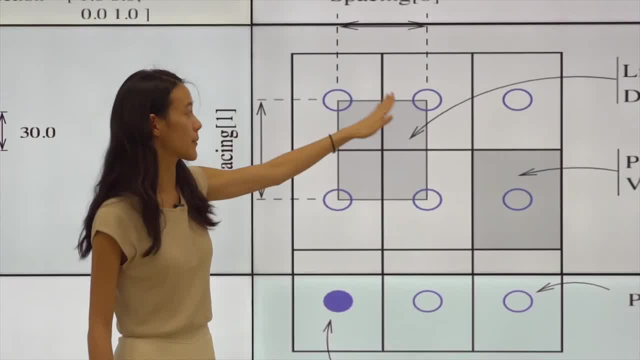 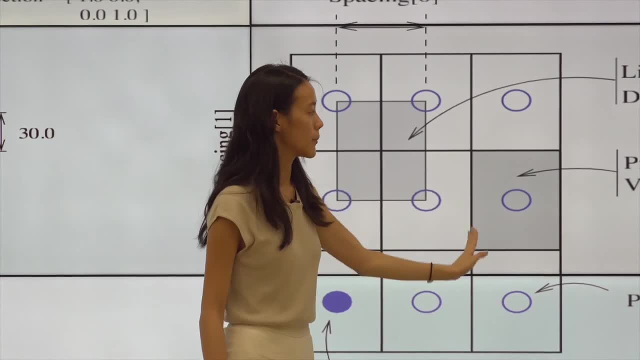 region of of the pixel width of the image, is that we're going to be looking at the middle part of the pixel region, so what we're talking about is in between each of these things, and so, for the pixel coverage, a lot of times it's the entire pixel, so the box that we see, each of these are pixels, and 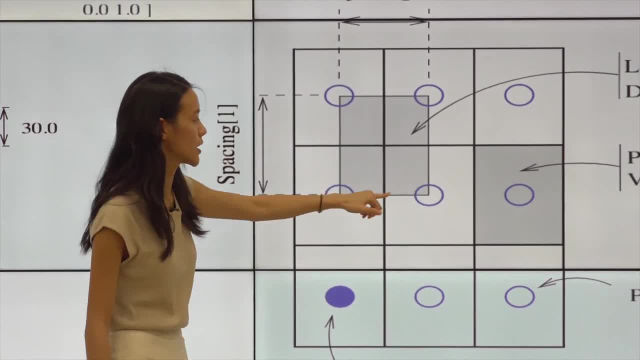 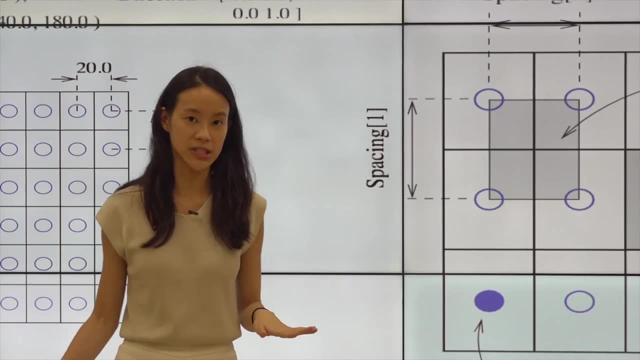 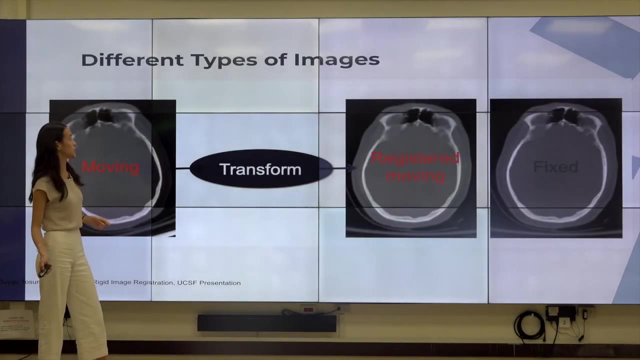 these are pixel centers, but when we're talking about interpolation, it is between the spacing, that is, between the four neighboring pixels that we'll see, or the four neighboring pixel coordinates or origins that we will be seeing, and so one thing to know as we're reading the images is that there are 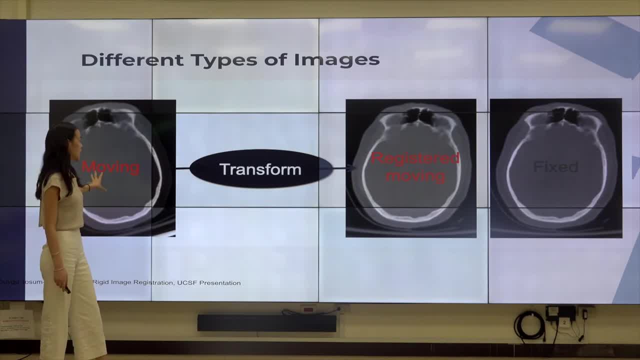 two different kinds of images when it comes to registration. so there is a moving and there is a fixed image. so I'd like to refer to the fixed image as a reference image, something that the algorithm, or the registration algorithm, refers to every single time it is trying to register that moving image. so, as we can see in 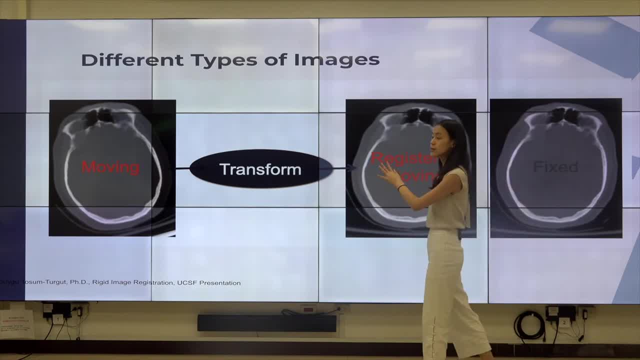 this diagram. what we tend to have is that moving image and it goes through these multiple transformation processes before becoming registered with that fixed image. so what we would end up seeing is this original moving image being rotated and going through all these processes so that it ultimately ends up looking very similar, or maybe even exactly the same thing as the fixed. 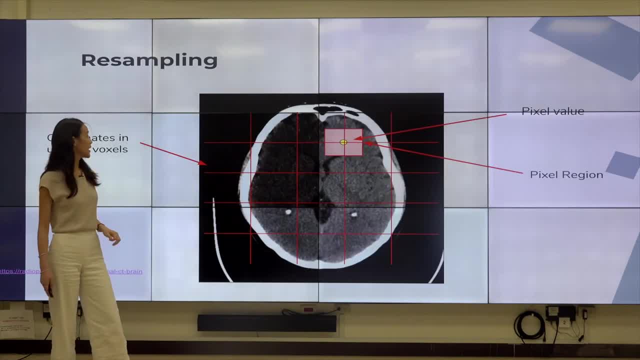 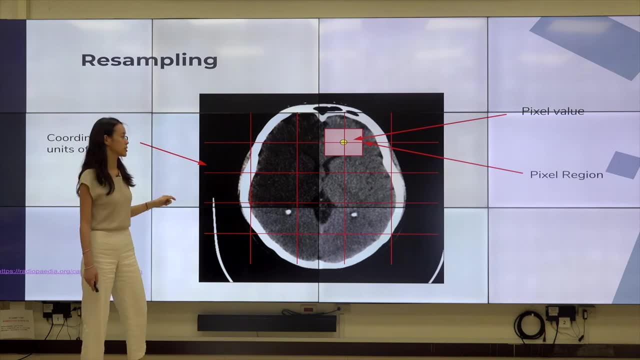 image or the reference image, and so one thing to know, as we're talking about resampling, is let's kind of jog our memories back onto how we defined that grid that we were looking at at the two slides earlier, and so these are in coordinates of voxels, units of voxels. so, as we stated before in previous lectures, voxels. 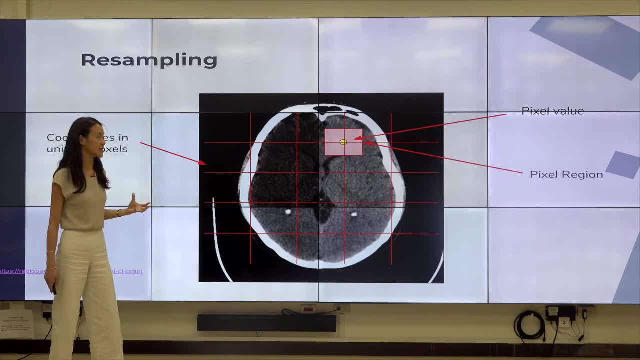 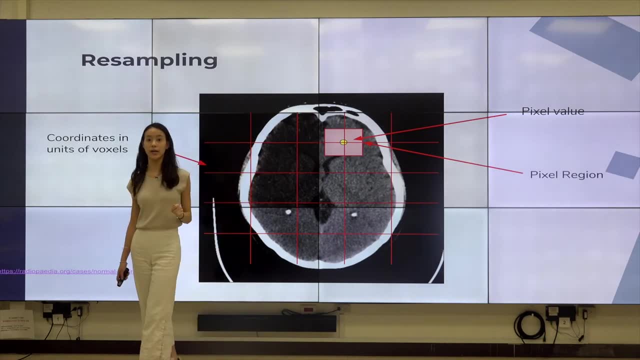 are in terms of a 3D kind of sense of image analysis, and so one thing to note is that we're looking at the pixel value, which is that middle point, and the pixel region, as we're talking about resampling. so this is just a redrawing our memories in terms of how resampling occurs. 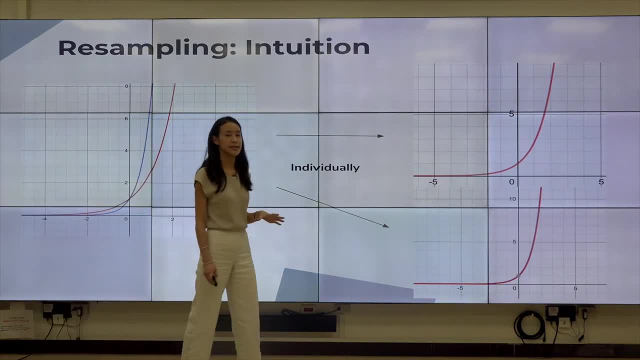 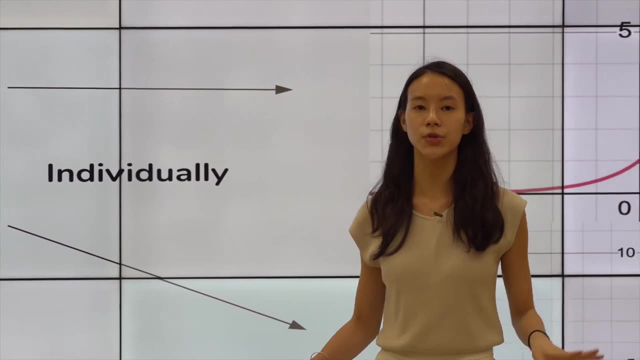 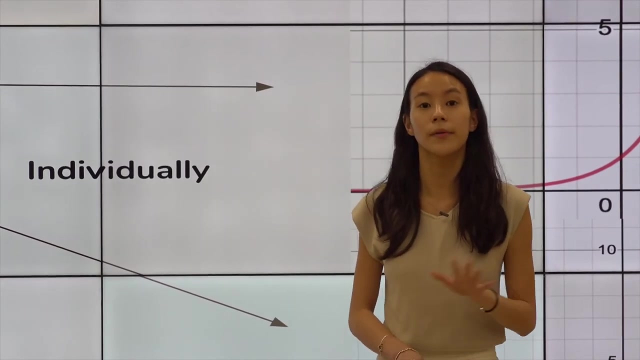 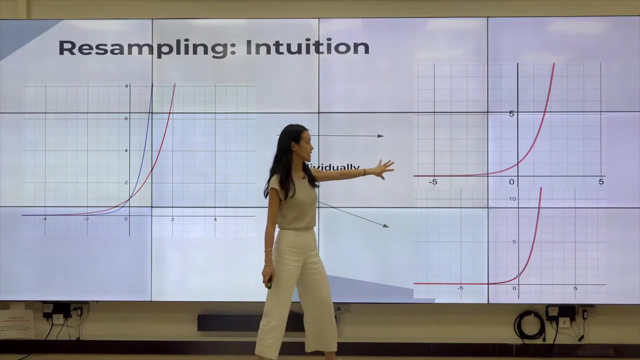 so the entire idea behind resampling is that we're trying to create new points in order for the entire image or in order for the two images- the registered and the fixed image, or the moving and the reference image- to become more comparable to each other. so the way that I would like to see this is, for example, in two different situations. so let's say: 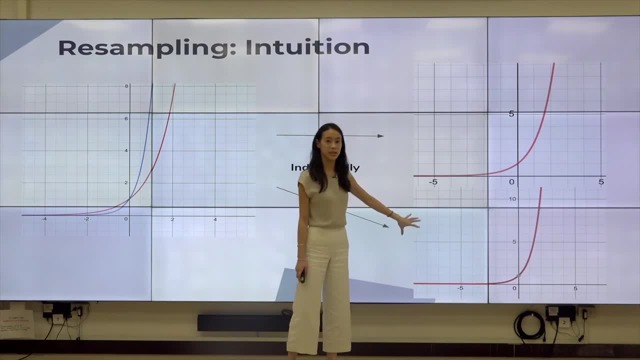 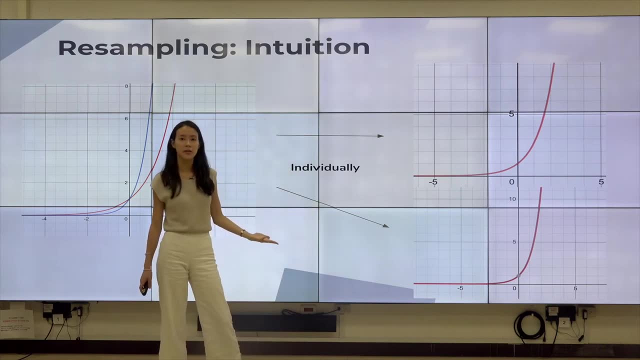 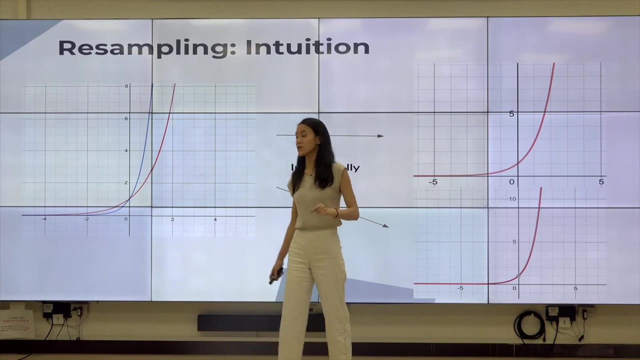 that this is the fixed image and this is the moving image. so, looking at these two graphs, we can see that, in terms of spacing, they're similar. they're very, very similar in terms of shape, in terms of a lot of things. however, in reality, it's actually very different. as we can see on the left side, they're very, very different when you're. 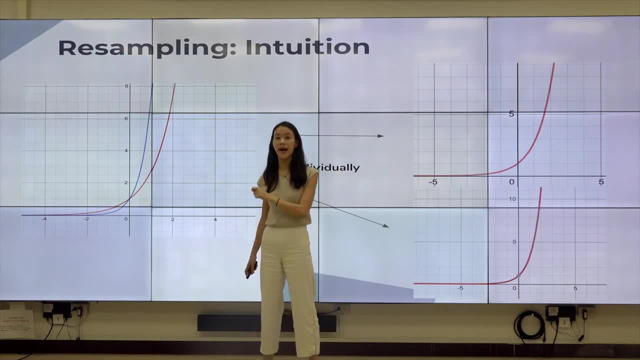 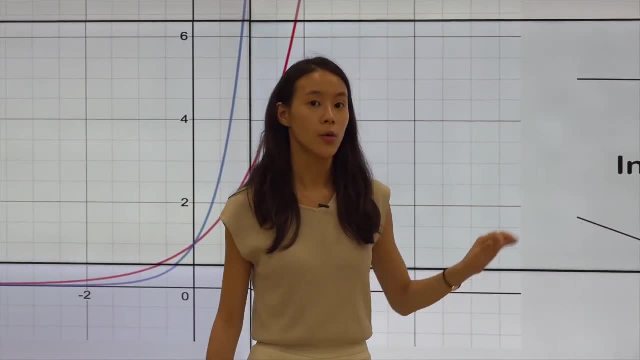 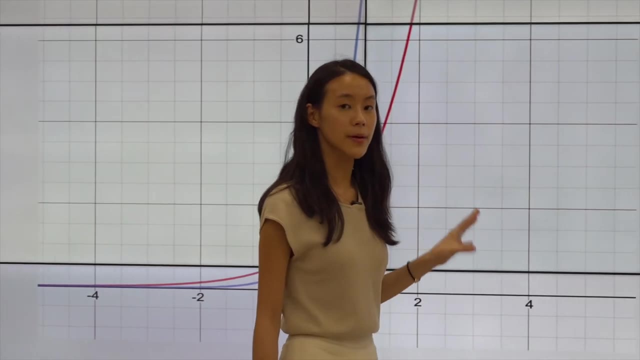 looking at them, one is actually increases exponentially faster than the other, but it wasn't differentiable when we split them up into two. so this is where resampling becomes important. we're having them both, or both of the images, on the same scaling, on the same grid, so that they 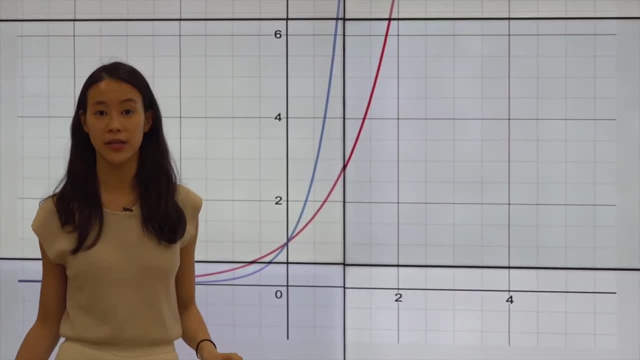 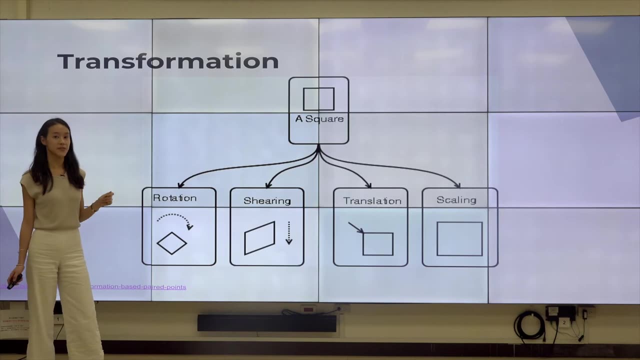 can become more comparable, so that registration is a lot easier for the, for the entire algorithm itself. and so, going on briefly to talking about transformation, for the sake of our purposes, today we're only going to be focusing on linear transformations, which include rotation, sharing, translation and scaling, and you can see what each of these transformations mean by comparing. 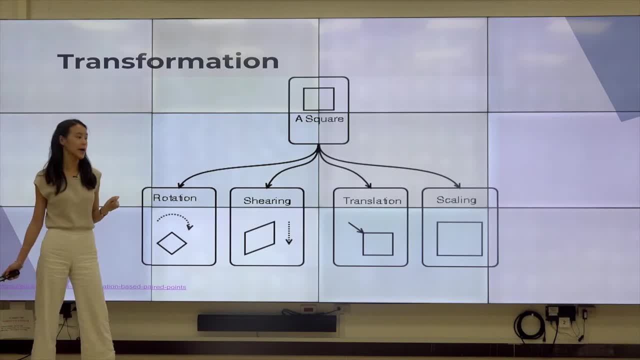 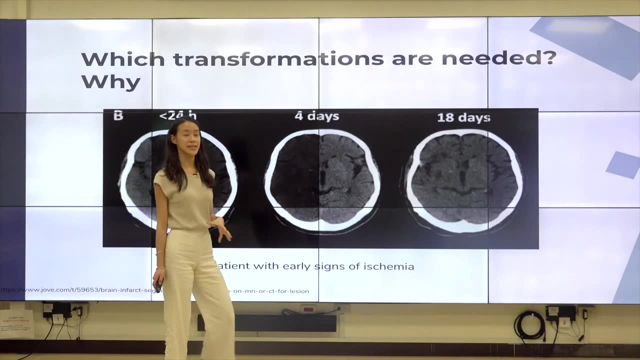 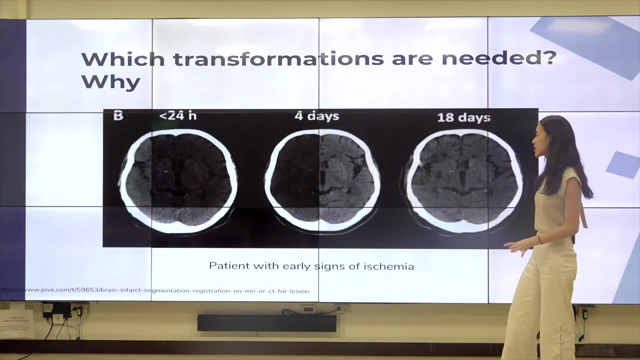 it to the original, the original structure, which is the square, and so one thing that I would like to ask you guys, after everything that we've talked about, is what kind of transformations are needed and why so, looking at these images, which is a patient with early signs of ischemia, what kinds of transformations do you guys think you would? 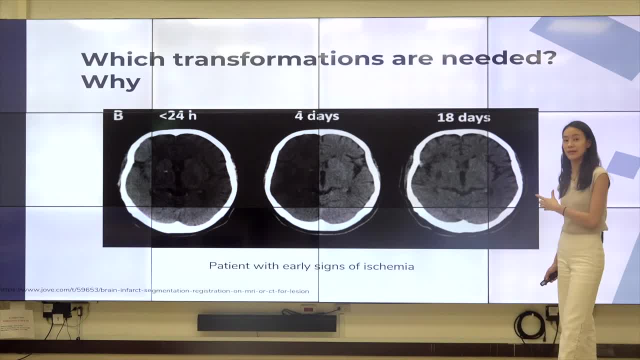 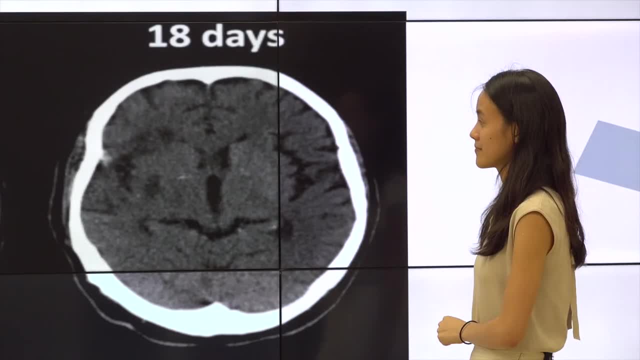 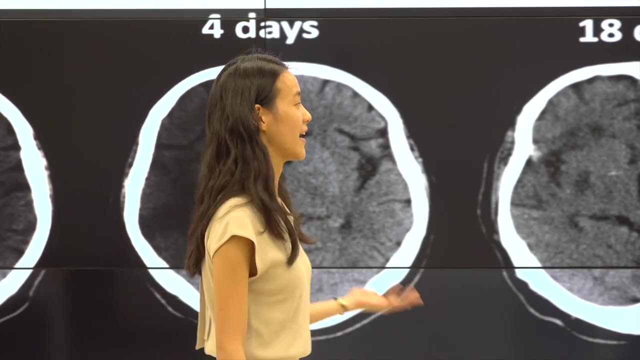 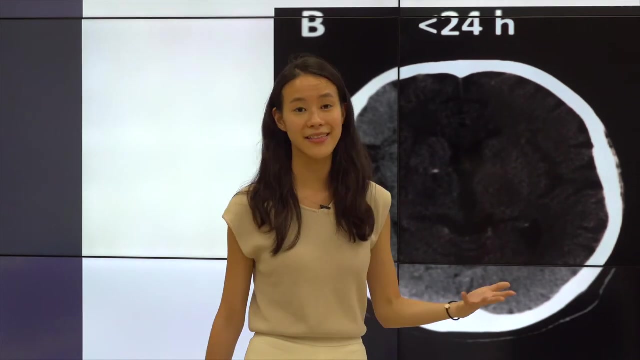 need in order to compare these three images- which is something that I'm hoping that you guys remember- which is the same patient, but different times. so, honestly, there's no right answer to this. you can compare it in any in any single way. so we can say shearing, we can say rotation, we can say scaling, we can say anything, basically. 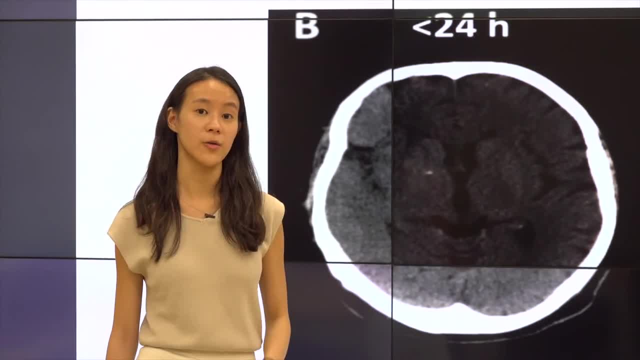 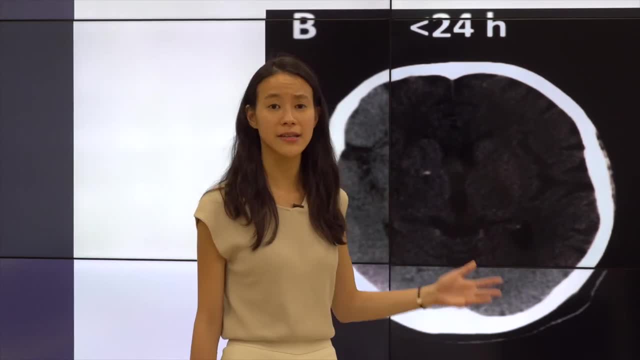 there is no right or wrong answer with our own eyes. so with the human eyes it is very biased, because what we may see may be different from what someone else may see. so I may say like shearing or scaling, but someone else may say rotation and sharing. so 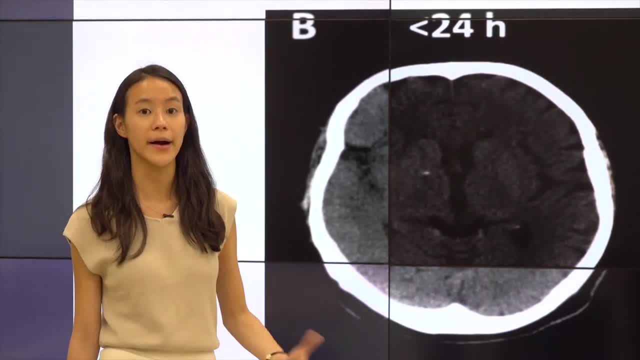 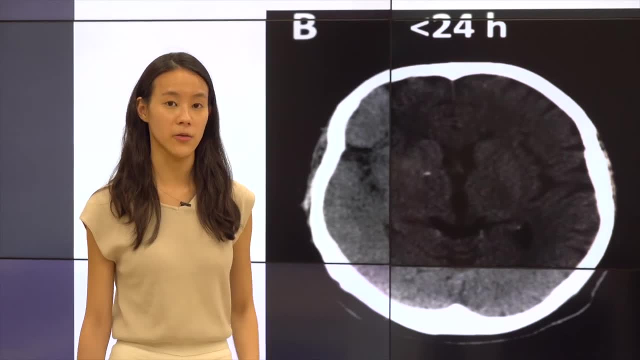 When humans compare these images, it is very easy for it to become biased when we're trying to register. This is why it's so important for the computer to come in where they have a set algorithm or a set rule. You can think of it as a set, a number of rules where they go through a number of steps. 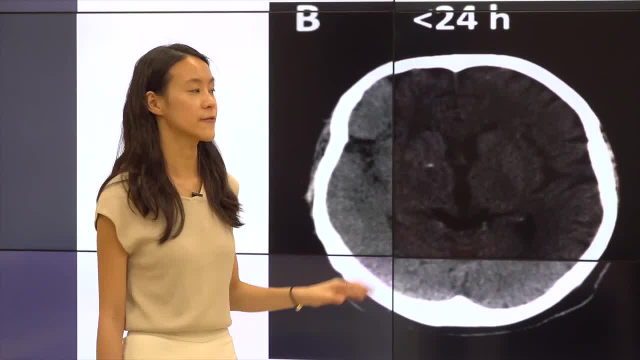 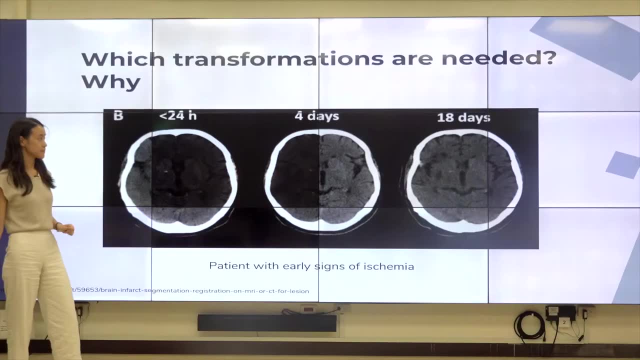 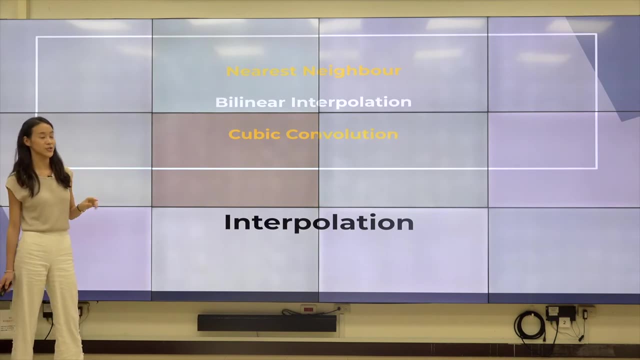 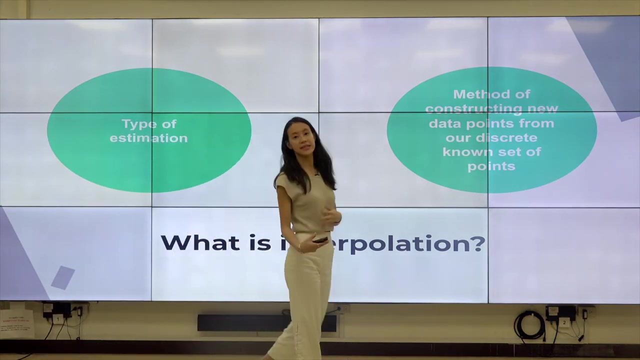 that they go through. that becomes more standardized, for these images to become more registered. One computer can help us decide on everything together. Talking about interpolation, it includes three different kinds that we usually see. What exactly is interpolation? I would like to think of it as a type of estimation. 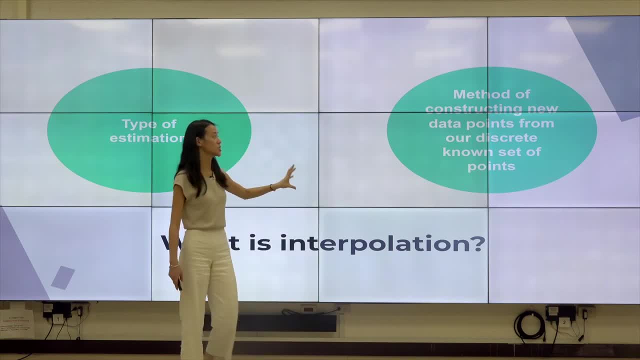 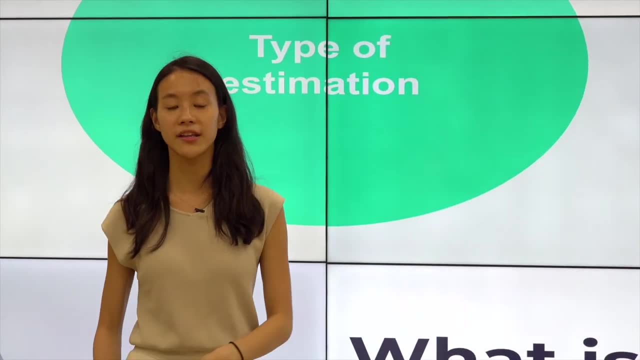 Interpolation basically allows us. it is a method of constructing new data points from our discrete known set of points. In this case, it may be, for example, if we had 1,000 pixels on one of the images, such as the reference. 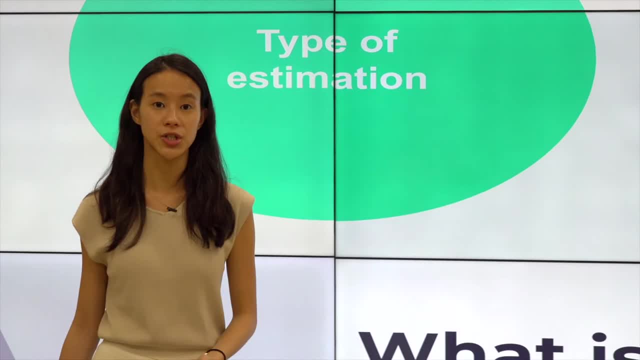 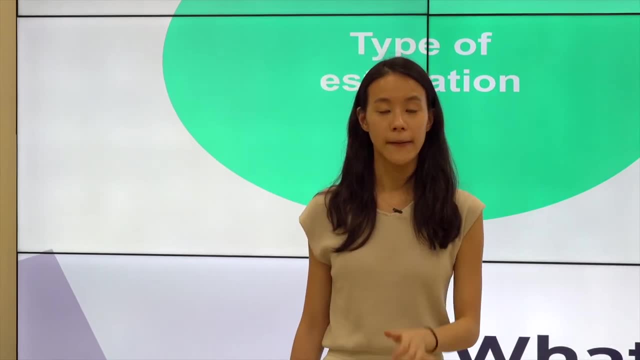 The reference image had 1,000 pixels and the moving image only had 500.. What we would need is interpolation so that we're able to create an additional point between the two points for that 500 pixel image, so that we can create 1,000 pixels, so that these 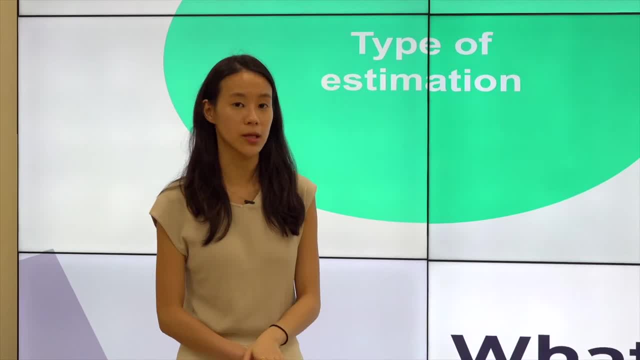 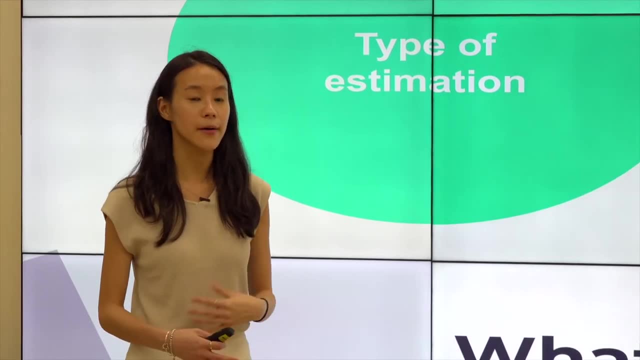 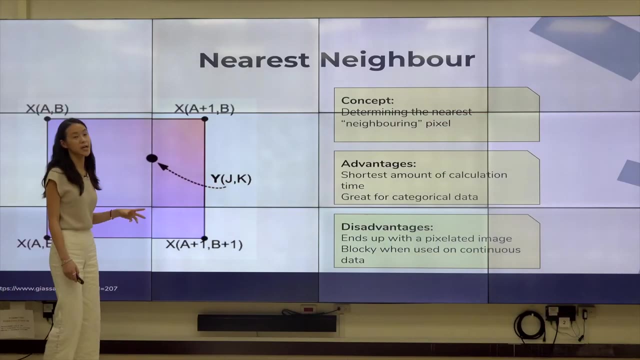 two images can be registered together or can be compared together, as we saw in resampling, where we need it, on the same grid. That's the entire process, or the entire need or function. Going on to talking about nearest neighbor, which is the simplest interpolation method, 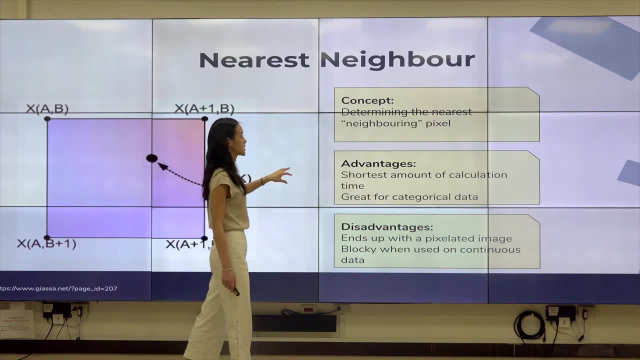 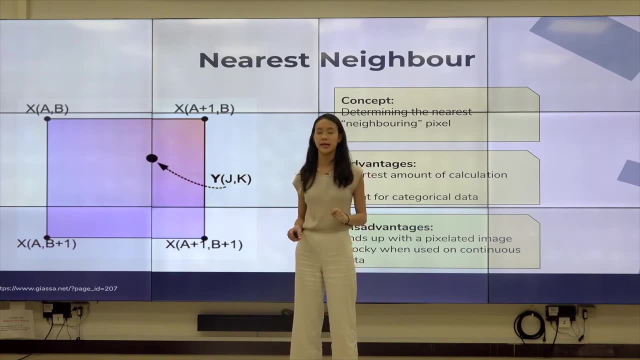 that we have ever come across. The concept behind it is determining the nearest neighboring pixel. The way that I would like to see it as: imagine yourself, close your eyes. imagine yourself standing in a room where there are four corners to that room, very distinctively. 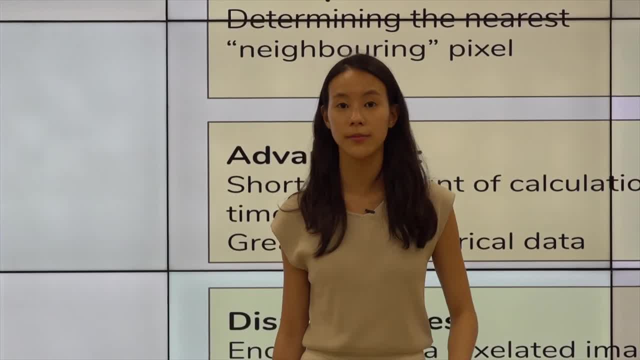 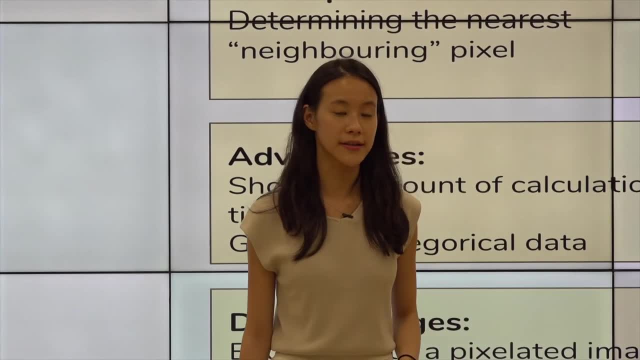 Imagine yourself standing near the door which is to the left side of the room. It's the bottom left side, if we're looking from above. What we would see with this bird's eye view is the fact that if we're standing near the door which is on the bottom left, what the nearest neighbor algorithm does is that it. 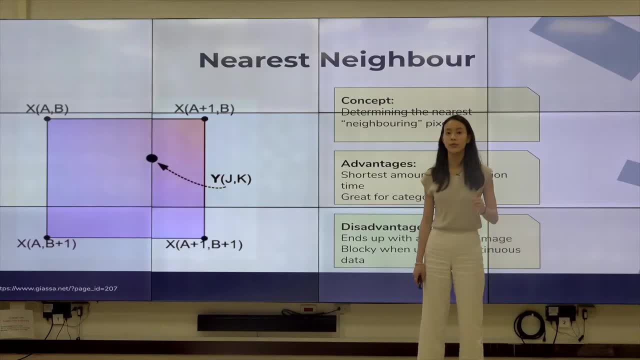 interprets your point as that door point. We would define ourselves as that point, without consideration of anything else. This is why I told you this is the simplest thing. Wherever I'm closest to, that would be the point that I would define myself as. 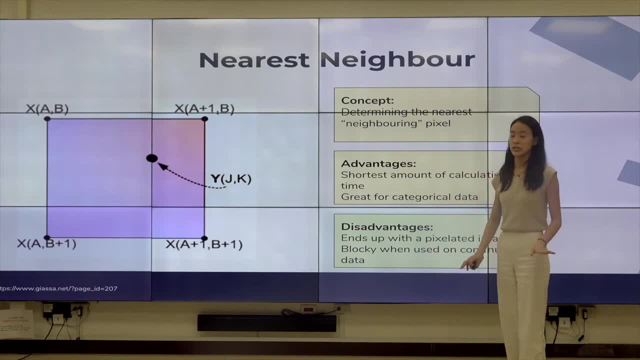 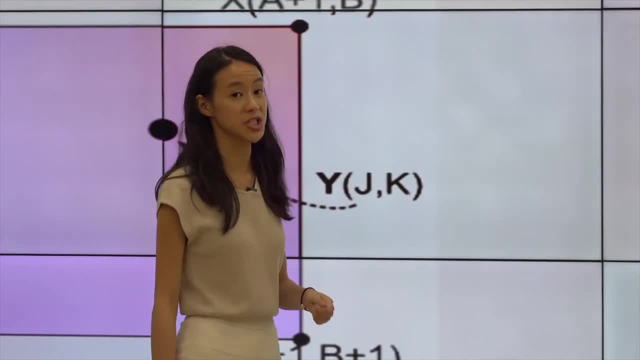 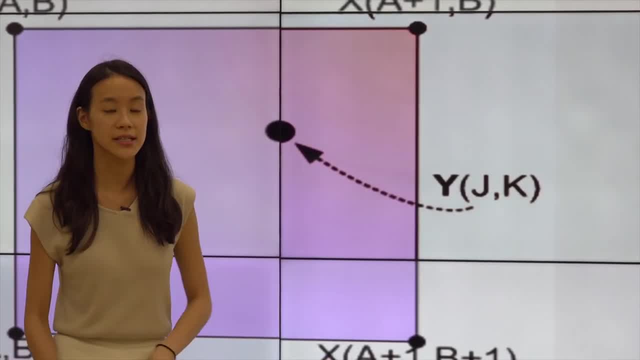 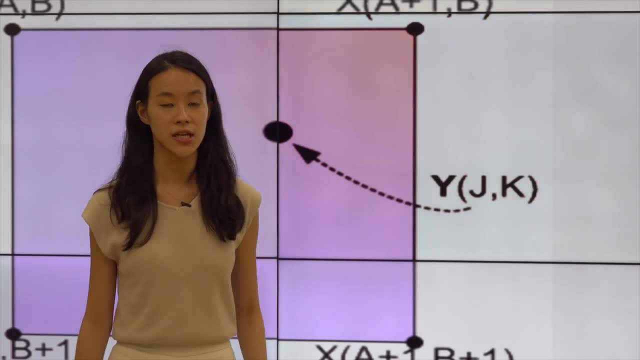 age Mexicans and yet find a better answer than the one that I've shown. These two understand best job ESAS. to infer for a police officer is to apply this to their job ESAS. is that both they should ride into the club every day while you're moving to? 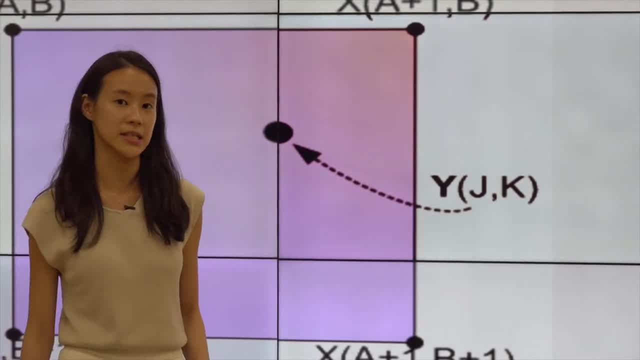 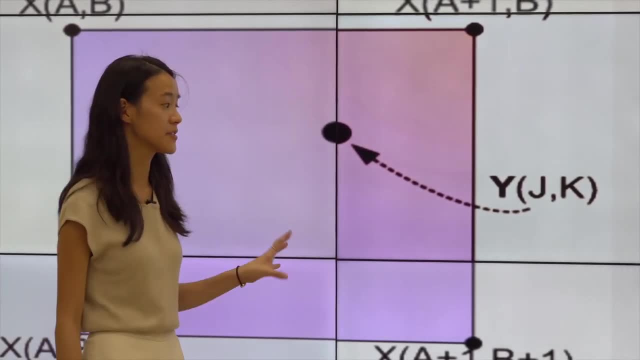 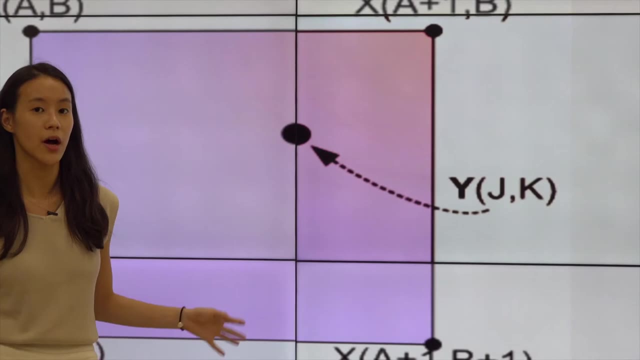 easy to split up without any other consideration or waiting system. It is very quick and just very. it's a very good decision process for categorical data. The disadvantages to this is the fact that it ends up with pixelated image and it is very blocky when you're using it on continuous data, as we will. 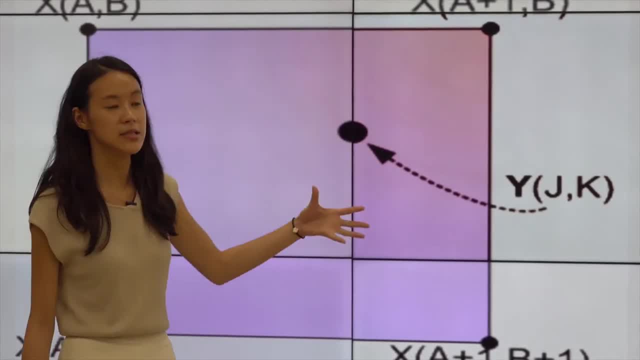 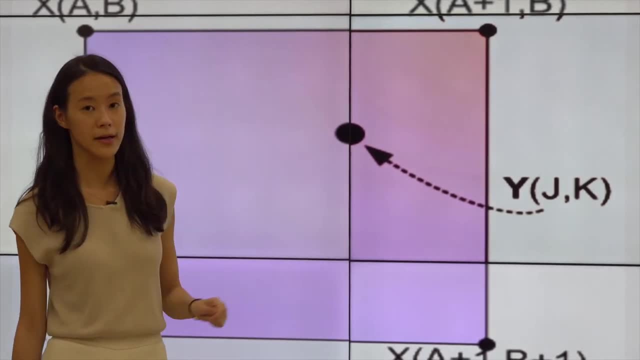 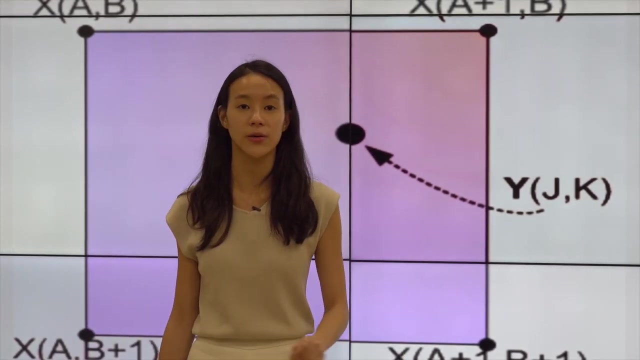 see later in a visualization process. So this makes sense, because we're not considering any other parts of the room except for the closest corner, and so that's why we end up with a lot of pixelated images. a lot of times There's no consideration of any grey numbers or any numbers between 0 and 1, it's 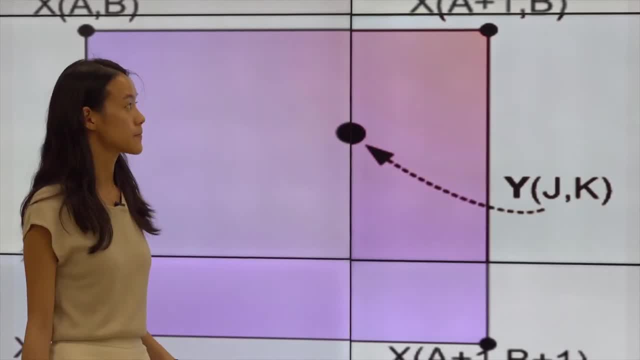 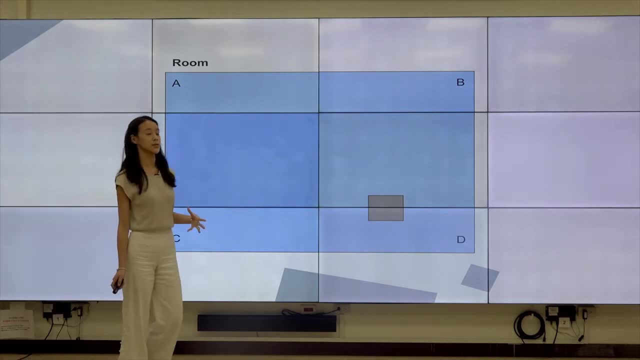 either 0 or 1, no decimal point, And so this is exactly what I was talking about before, and so just to summarize what I was talking about for nearest neighbor, imagine yourself on the bottom right corner in this case, and so if you're- 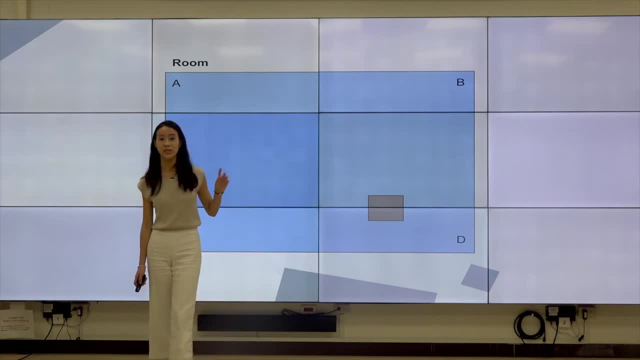 closer to D. what nearest neighbor does is that it doesn't consider A, B or C adults. all All it considers is D, because you're closest to that, and it immediately categorizes you into D, nowhere near A, B or C. Bilinear interpolation is a better. 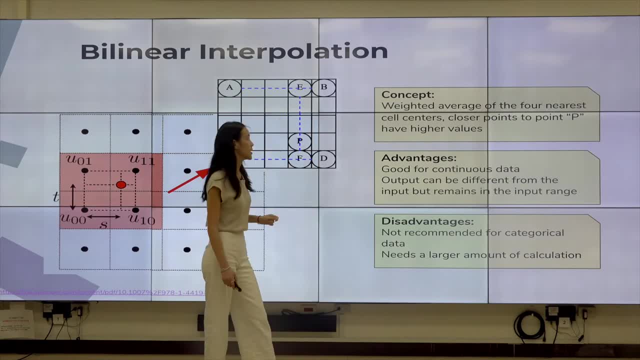 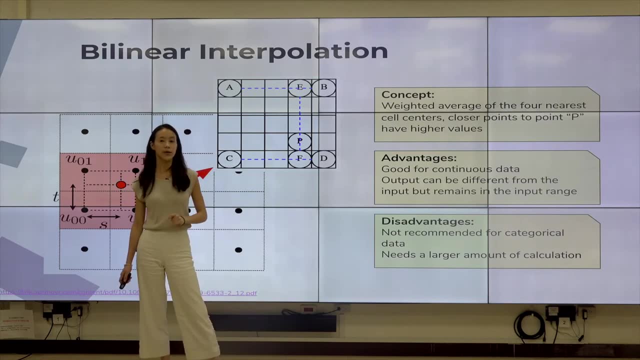 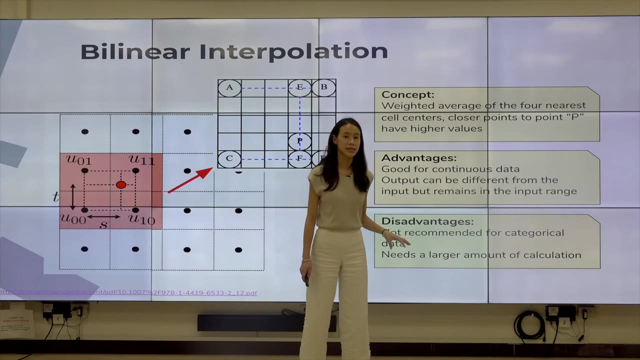 method, or you can think of it as a step-up method from nearest neighbor. So the concept of this is that you have weighted averages of the four nearest cell centers. closer points to P would have higher values. So in the case of the room as we were talking about before, with the A, B, C and D, if you're closer to D. 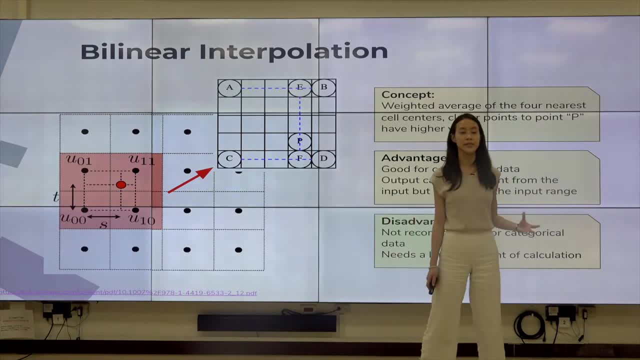 then that means that the D would have a higher weighting or higher value, since it is the closest corner to P. And then, obviously, the B area, which is the furthest away, which is diagonally from where you're standing right now, would have the lowest value because it is the furthest away from your point right now. 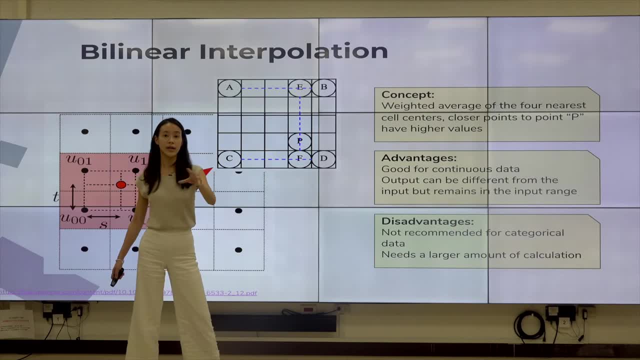 So that would have the lowest weighting. And what when you end up having is adding up all these values, you're able to determine your spacing relative to all four points or all four corners of the room. So the advantage of this is the fact that it is good for continuous data and the output. 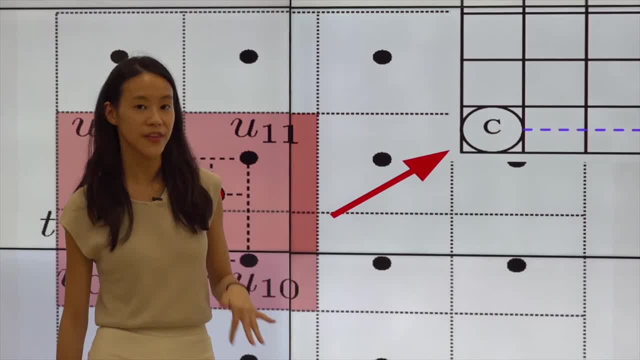 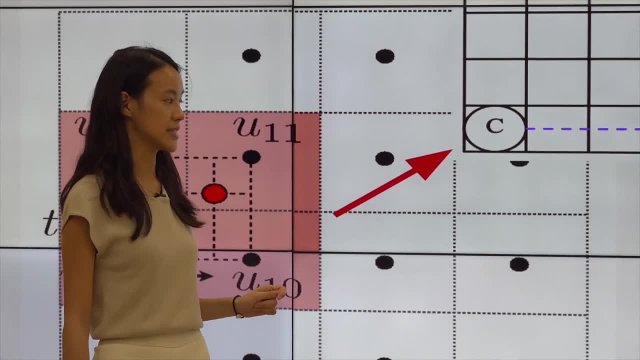 can be different from the input, but it remains within that input range that we originally had, which we will show you or you will see in the visualization later. And the disadvantages to this is the fact that it's not recommended for categorical data and you can think of this as if you're trying to categorize. 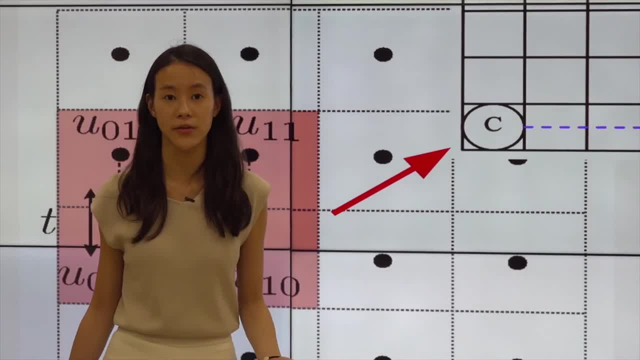 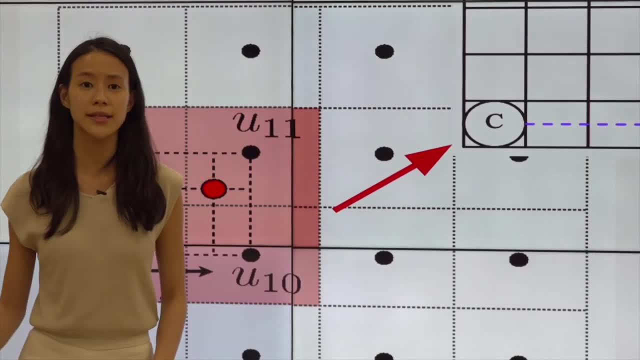 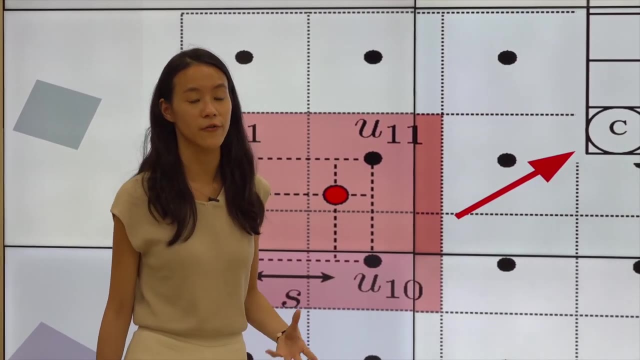 yourself if, going back to that Oreo situation, some people may argue Oreo is actually very healthy, it's not as high in sugar or whatever some people need and maybe say they may categorize that as healthy data and so in that situation we would know that it's very difficult for us to have all these different. 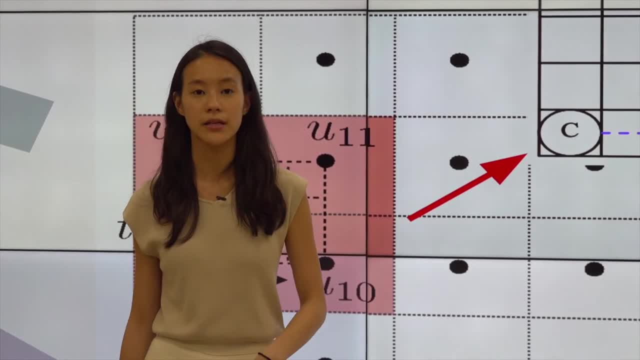 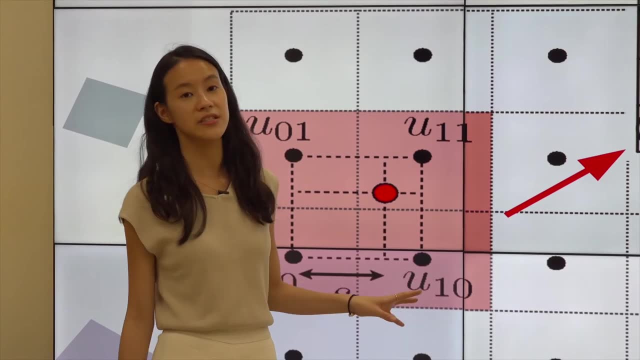 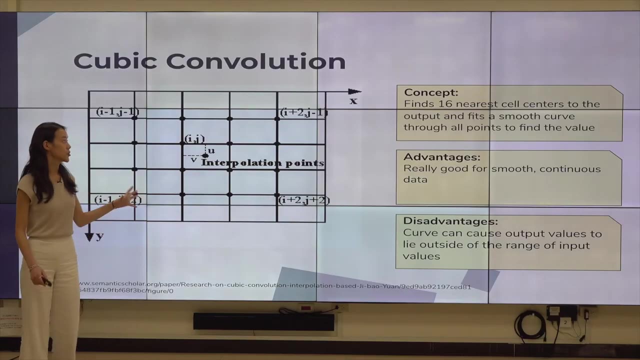 weightings, for us to be able to determine something that can be clearly or very easily categorized into one section without further considerations of other factors. And another disadvantage to this bilinear interpolation is the fact that it needs a larger amount of calculation. So, going on to the cubic convolutional method, I would say that this is a step up, a 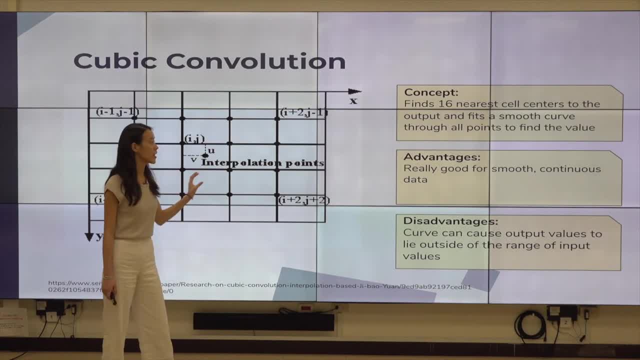 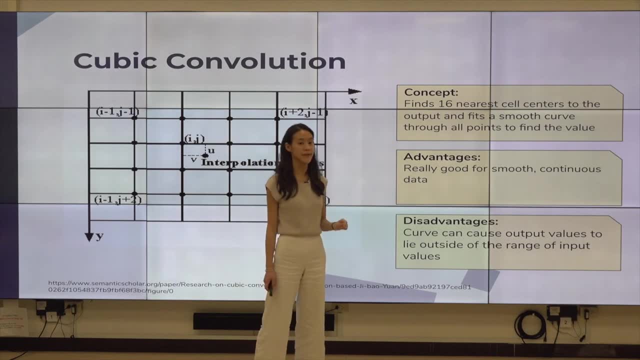 further step up to bilinear interpolation, and the concept of this is the fact that you're finding 16 nearest cell centers instead of 4 to the output and fits a smooth curve through all the points to find the value. However, the advantages of this is the fact that it's really good for continuous and smooth. 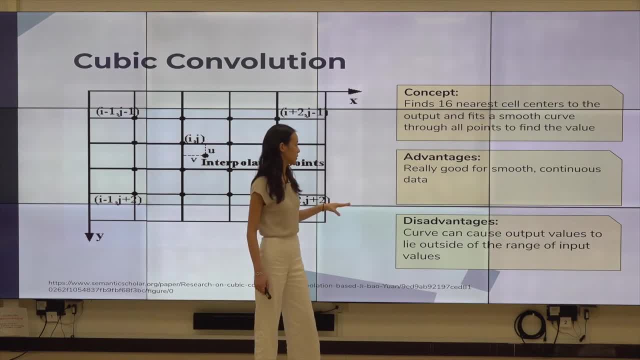 data. However, the curve can cause a lot of outputs to lie outside of the range of input values or the input range, and one thing to note about this is the fact that it is also very time-consuming to compute. So, since there's a lot more data, 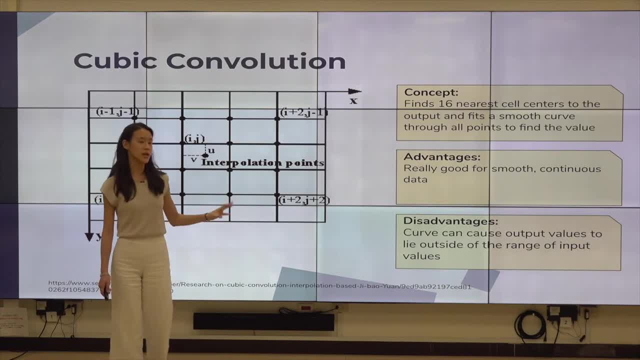 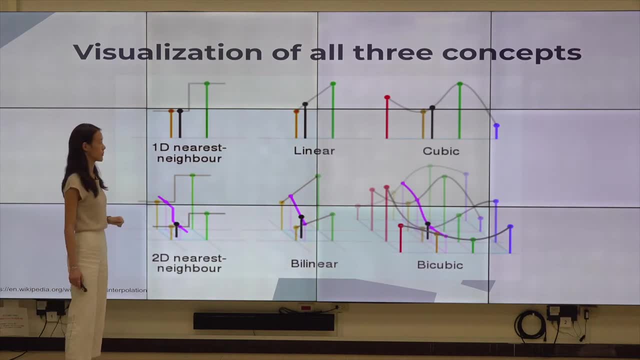 going in. there's a lot more computational stuff that it needs to go through, so a lot of times we wouldn't see this method used as much. So, going on to talking about the visualization as I was talking about before, there's a reason why the images become more pixelated, as we can see in the 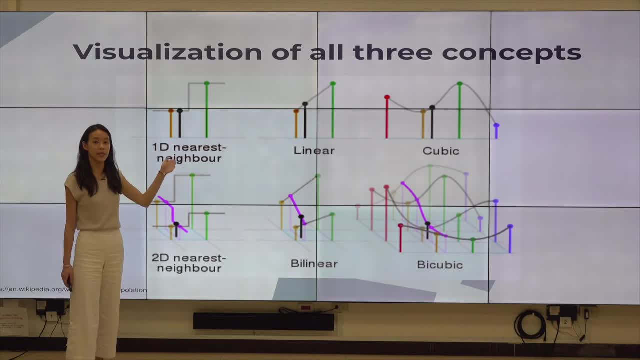 situation. It is blocky because you're taking a step up from each step. so there's no data in between these two. So, as I said before, this may be 0 and 1.. There's no data between that 0 and 1, so there would be some kind of unknown data. 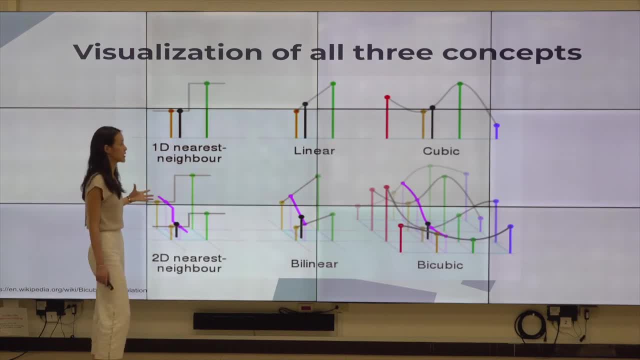 between these two, which makes the entire image more pixelated. On the other hand, when it comes to bilinear interpolation, what we meant by the smooth or the output range becoming or staying within that input range is- you can see this line here: 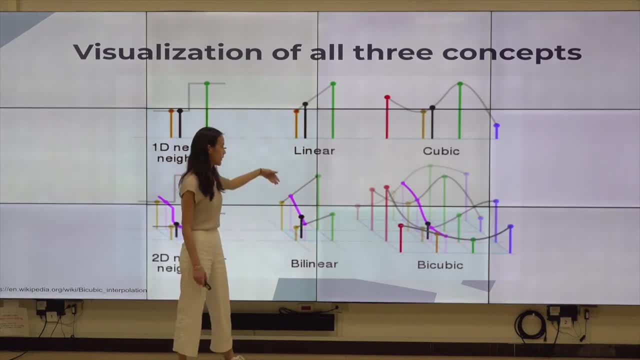 So these two lines are at different heights and by combining or connecting these two different linear interpolations, we can see a smooth line that is descending from that higher to the lower. So, as you can see, it's staying within that high to low range. 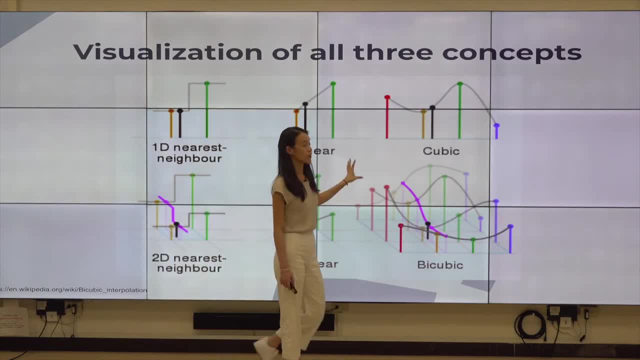 So any of the outputs are staying within. However, with the cubic convolution, as we can see here, what ends up happening is that you have that curve that goes up and then down, So that upward motion that you see here is already going outside of the input range. 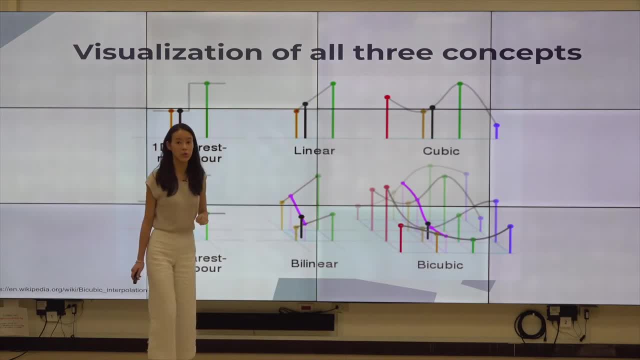 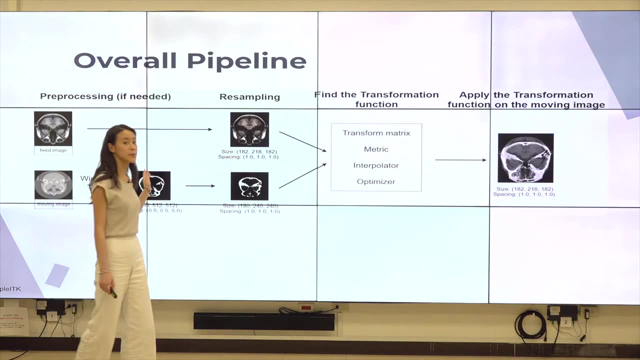 that we originally had And that was the disadvantage to cubic convolution. So, going on to the mathematical concepts of registration, So the entire pipeline or the workflow of registration, as I would like to explain here, is that we start off with the pre-processing. 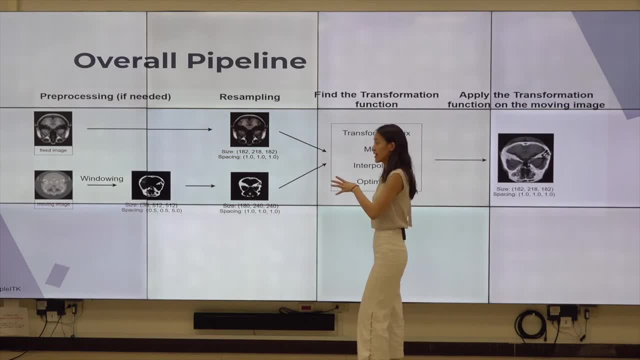 So if the image needs pre-processing, it would go through that process And, having that pre-processed image, we'd go through that entire resampling process that we talked about before, before going into the entire transformation process, which is the very first part. 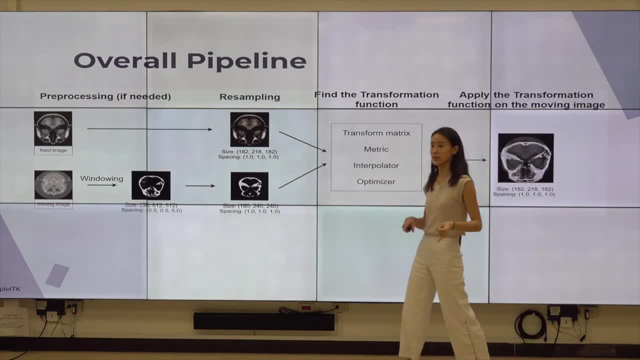 where we're finding the transformation function. So that would consist of the transformation matrix. It would consist of the metrics, the interpolator and the optimizer, which we'll explain in this section, And further details, And applying that transformation function to the original moving image. 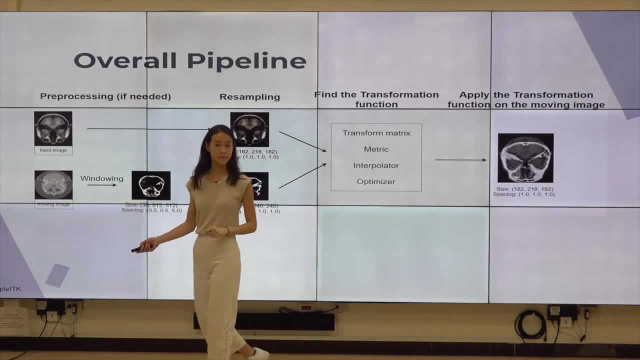 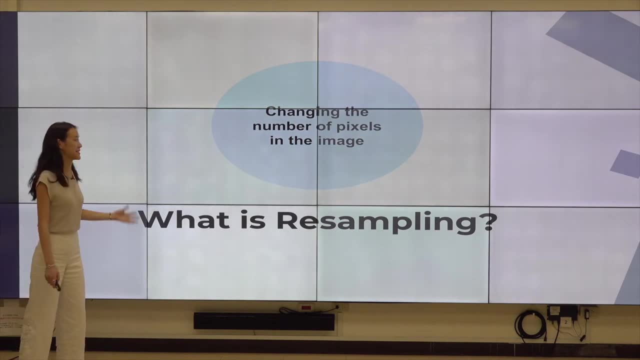 we would have this outputted registered image. So to reiterate what exactly is resampling- And the answer is already given to you guys, But just a reminder- it is changing the number of pixels in the image. So, as we explained before, 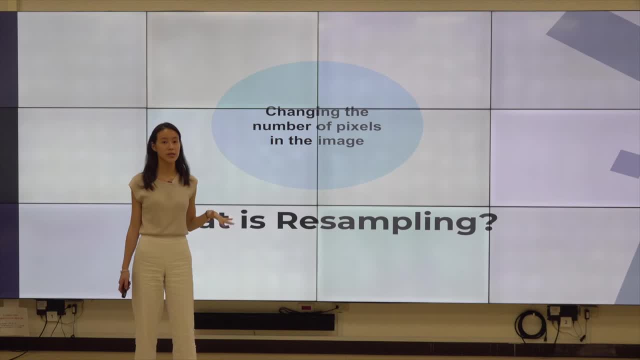 that 5,000 to 1,000 kind of idea or concept. that's what resampling is. We're trying to make sure that the number of pixels of the moving image is gonna be the same as the reference image, So that's easier for us to be able. 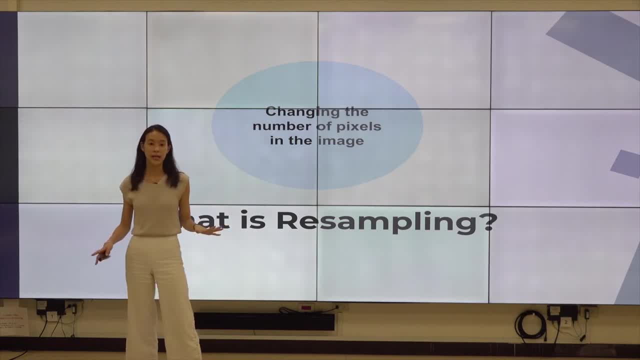 to register the two images together. So you're aligning- you can think of it as aligning the pixels or the points together in order to get our registered image. However, if we have different numbers of pixels, it's gonna be a lot harder. 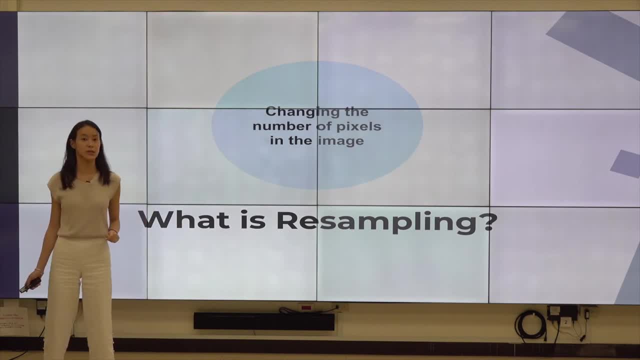 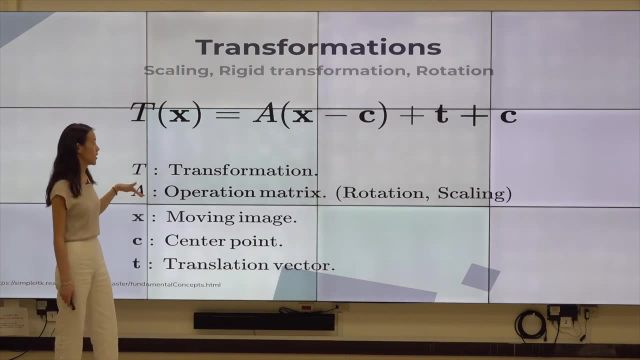 to be able to register the two images together, because there are no points that exist in between or to compare it with. So, in terms of transformation, this is the mathematical, this is a mathematical equation, And so this is the transformation function that we talked about before. 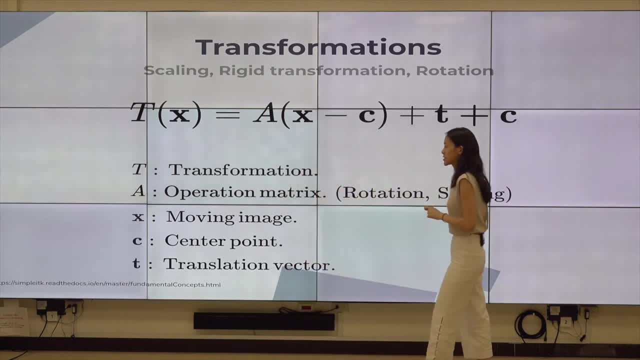 And, as seen here, the A is the operation matrix, X is that moving image that we were talking about, C is the center point that we have defined and T is the translational vector. So, using this, we would be able to find that transformation function. 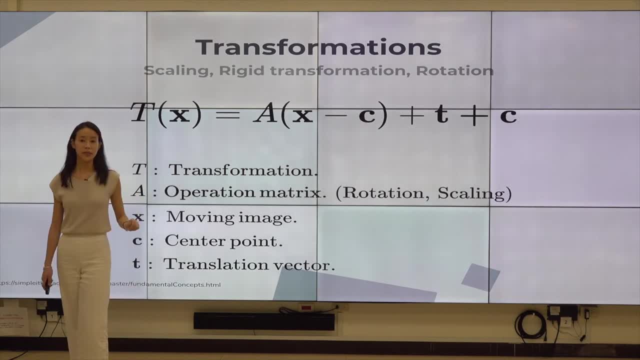 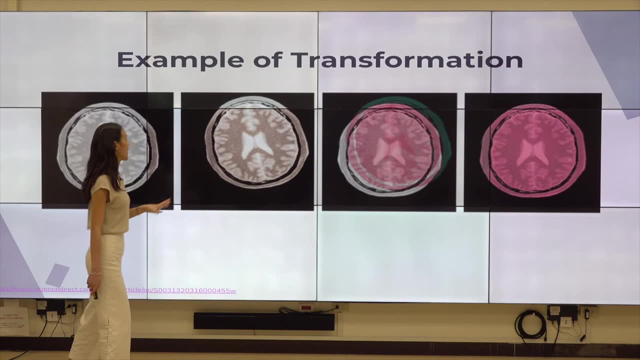 where we're able to put in our moving image in order to get our registered image, And so an example of transformation, as I would like to talk about again is: imagine we had this image at the beginning, And so what ends up happening is that it's not a direct method. 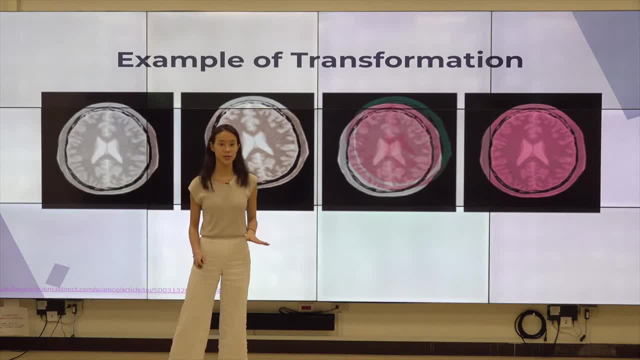 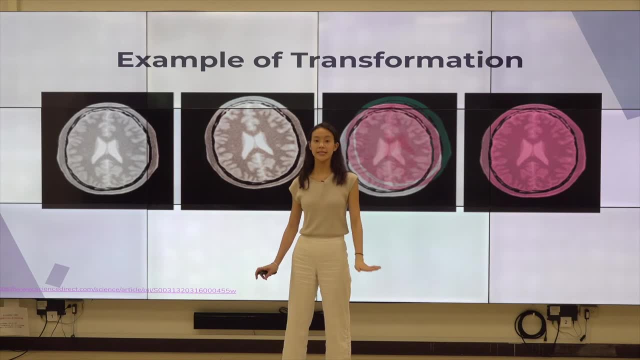 of just like having two things overlap on top of each other. So let's have a very good example right now. So everyone, close your eyes and put two hands out, And what I'd like you guys to do is to overlap them on top of each other like this: 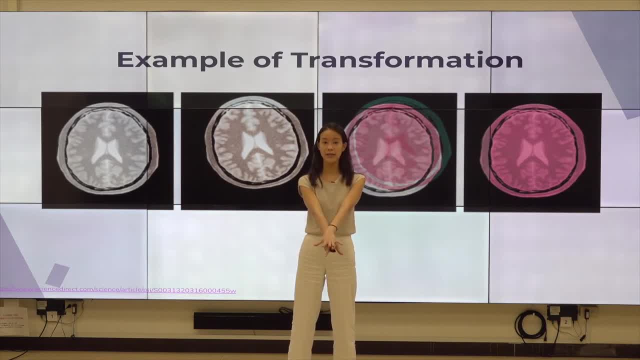 And with each of the overlap, with your eyes closed, I'd like to see. I'd like you guys to open your eyes and see how close your two hands were on top of each other, And so what you would learn is that I'm hoping with each iteration. 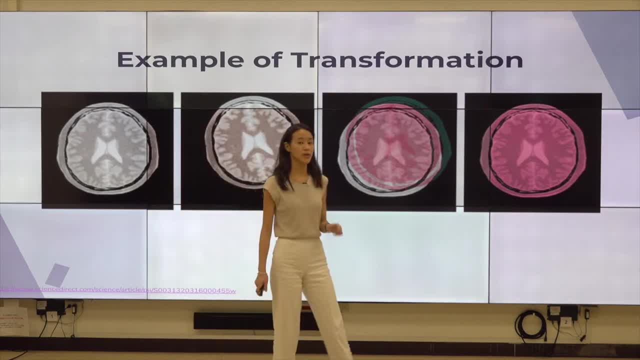 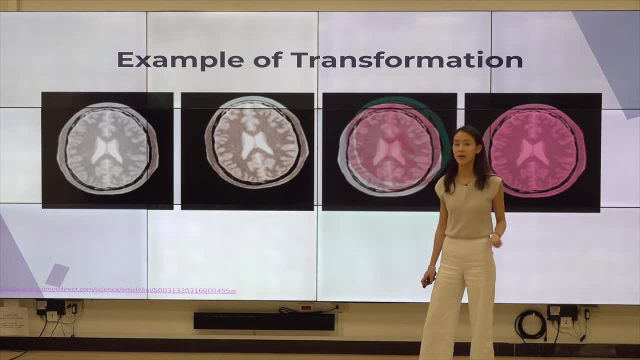 or with each try that you guys do take, you would realize that you get closer and closer to two hands exactly being overlapping on top of each other, And so that's the entire, or it's the exact same kind of situation when it comes to registration. 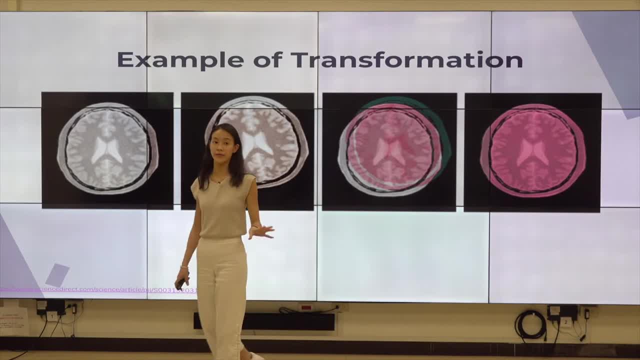 Or when we're trying to register a moving image, the reference image. So the bottom hand that we originally had when we're doing the hand situation would be our reference and the top would be the moving. And so it goes through each of these iterations. 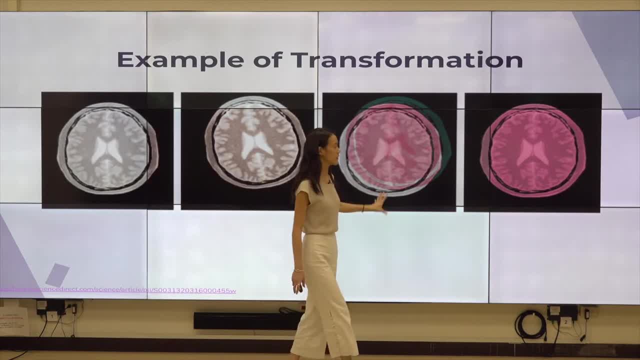 So it would move from like side to side to side until it finally has these two images that are overlapping each other, And that's when you know registration has happened, Same thing as your hand situation, And I'd recommend you guys to kind of do it yourself. 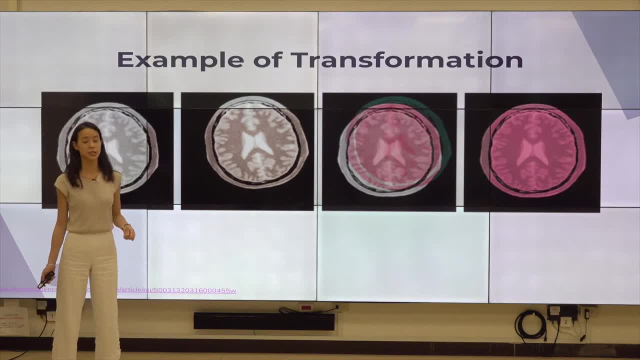 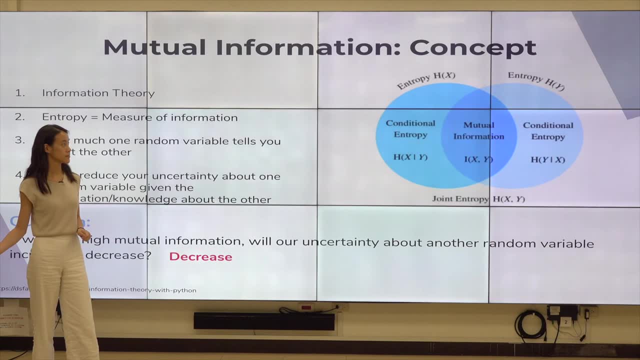 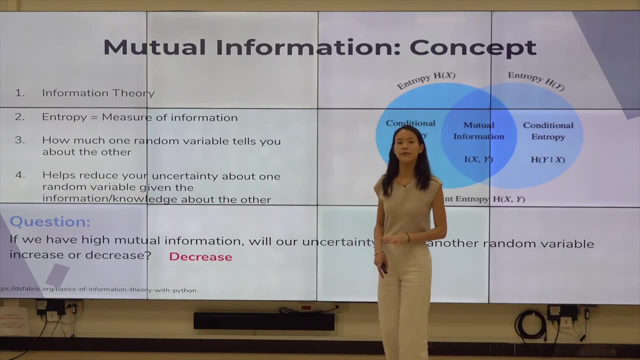 a little bit to understand what I'm talking about when we're talking about the intuition behind registration, So talking about the mutual information concept. So I'd like to kind of dive in a little bit deeper into the mathematical concepts behind registration, conceptually. So, mutual information is part of information theory. 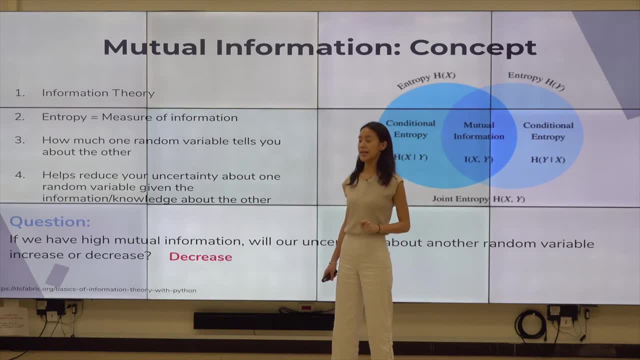 So one thing that I'd like you guys to remember is that entropy, in this case means measure of information. So in this case it doesn't mean that thermodynamic law that we've all learned. In this case it means the measure of information. 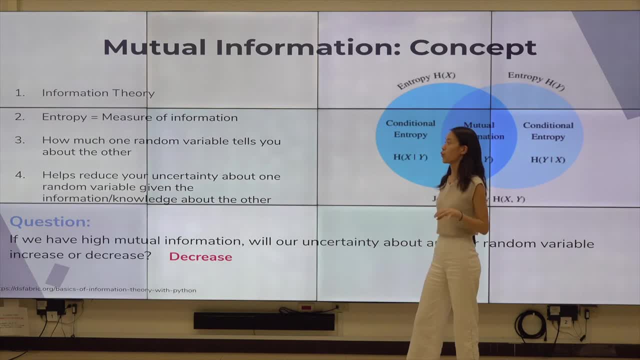 So mutual information allows us to learn how much one random variable tells us about the other, And so it helps us reduce our uncertainty about one random variable given the information or knowledge about the other. So what this actually means is: let's look at this diagram on the side. 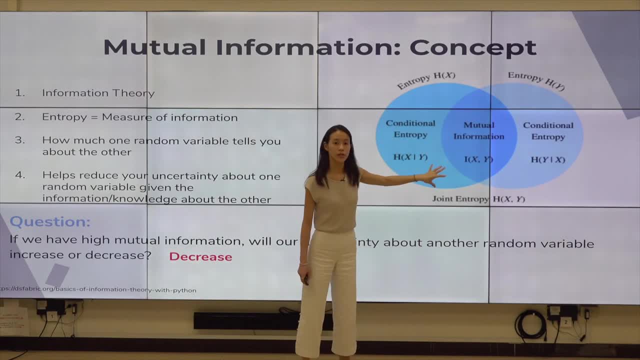 So having, let's just say, we had this original image on the left, or this original h of x, And so moving that h of y, by moving it closer together, we would know more and more about the right random variable, for example by overlapping it. 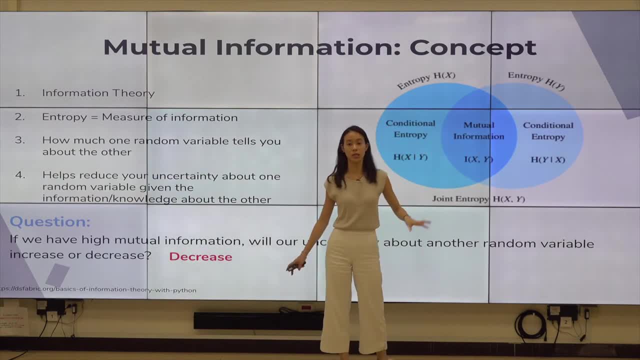 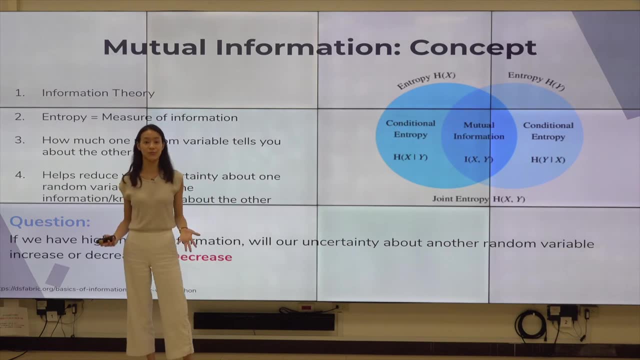 So this mutual information in the middle is where we're able to determine the two things. So let's take colors, for example, yellow and blue. So we all know adding these two colors makes green right. So imagine if we originally had blue as our fixed color. 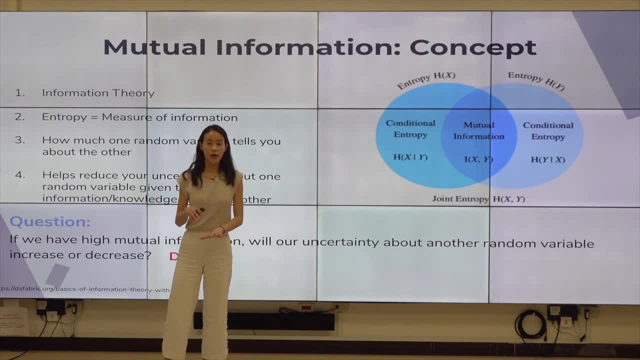 And we're trying to add the yellow in to create the green. So you would be starting off with a deeper green to begin with, right? So the more yellow that you add, the more the greener or the lighter green you get. And in this situation, 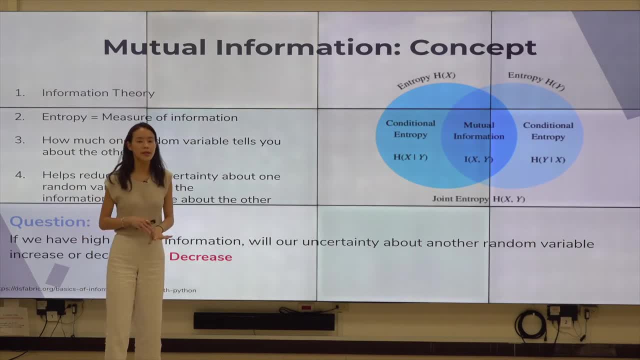 we can apply that to mutual information, where we know that the more yellow that we're adding, the more lighter green that we're getting. So we know more about the blue and the yellow, or we know more about the blue, depending on how much yellow we're adding. 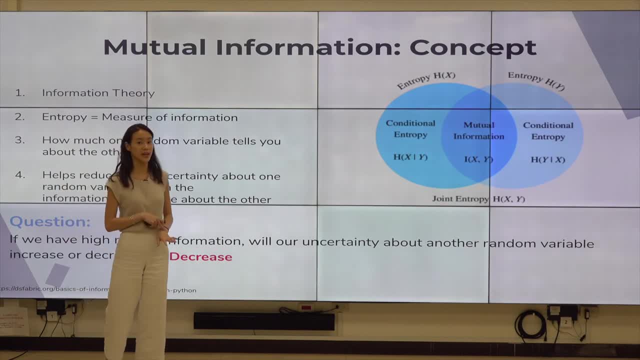 and the output that we're getting, so the mutual information that we're getting. So that's the entire concept of mutual information. So one question that I'd like to ask you guys is, if we have high mutual information, will our uncertainty about another random variable? 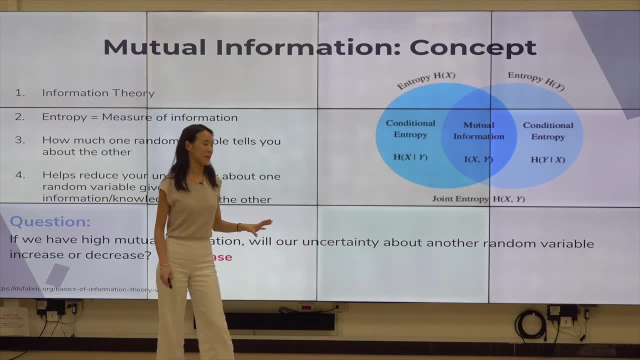 increase or decrease? So the answer's already actually there, but it would actually decrease And I would like you guys to think about why, depending or judging by what we talked about before. So, going back to it, going back to that blue and yellow situation, 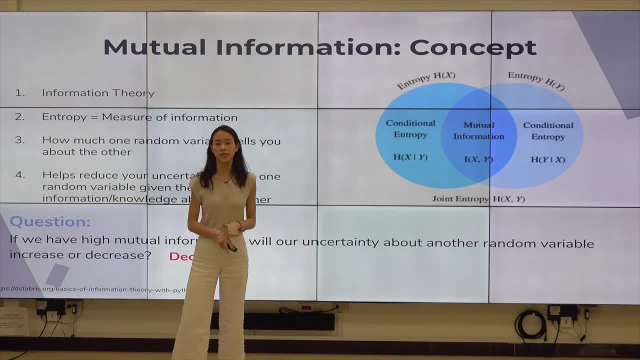 if we have more green or if we have more information about that green, then we could tell more about how much yellow we added or what kinds of yellow we added into that blue. if you think about it, If we have a more orangey yellow, 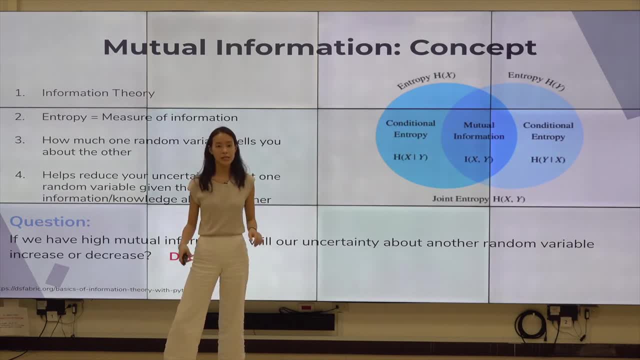 the green may be different from a more yellow kind of yellow. So, judging by the output or the mutual, the information that we get from the green, we're able to determine more about the yellow that we have inputted or the unknown yellow that we have inputted into the. 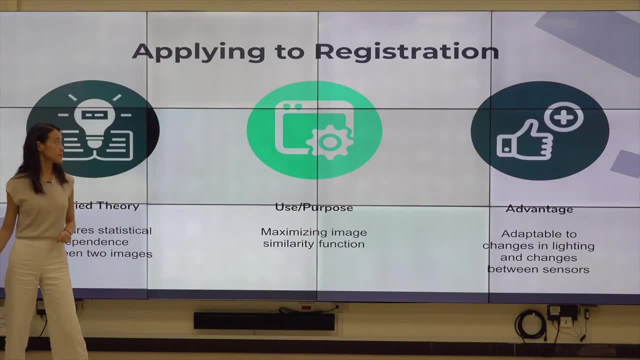 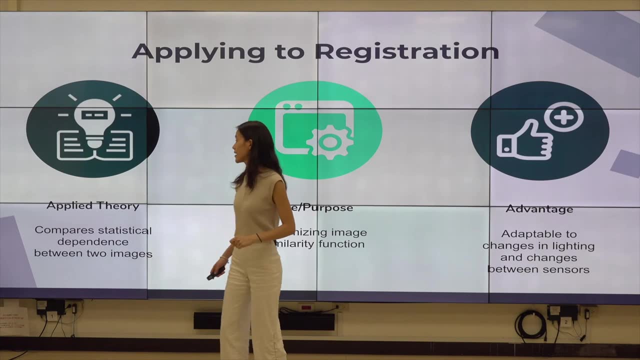 or that we've added to the blue color. So applying this entire mutual information to registration things that I would like to note is the fact that the applied theory is basically comparing the statistical dependence between the two images. So looking at the image of the fixed image, 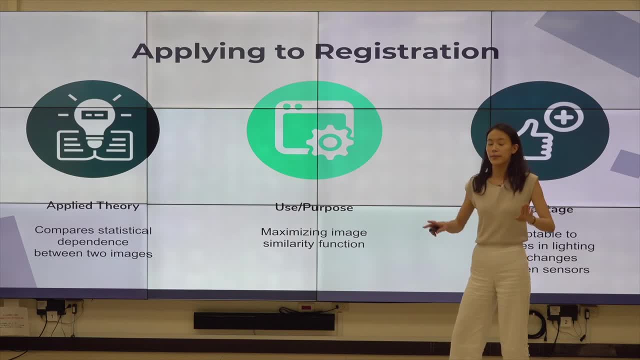 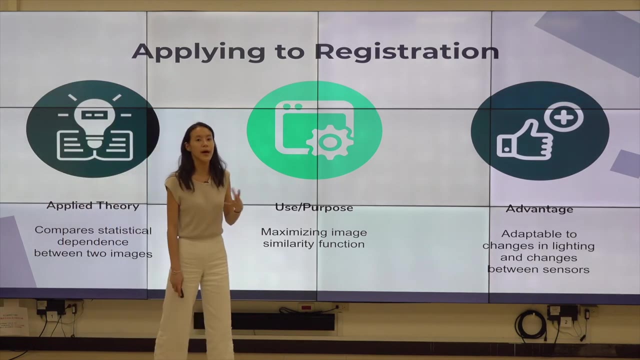 and the moving image. by applying, by looking at these two images, we're able to determine the mutual information between the two. The use and the purpose of this is the fact that we're maximizing the image similarity function. So one thing to know is that's not gonna give us the best. 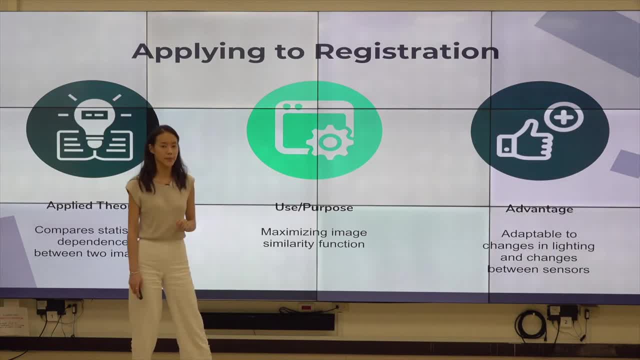 or it's not gonna give us a perfect kind of minimization, but what the algorithm does is that it ensures that we're able to get the optimal amount of information, and that's what we're doing: We're able to get the optimal amount of information. 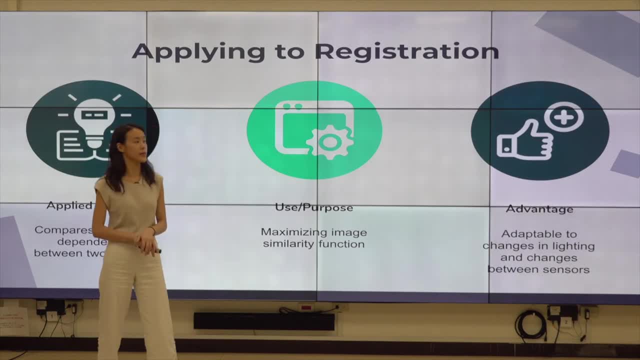 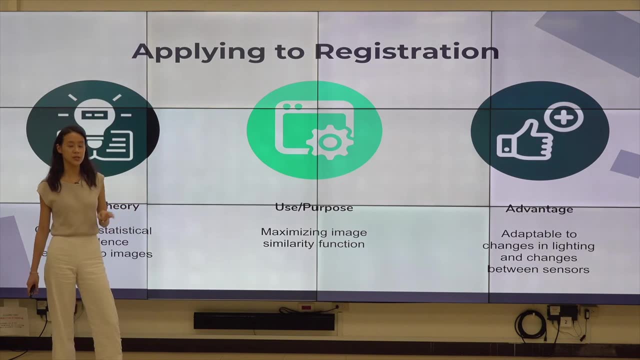 that overlaps, but definitely not the perfect kind of information that overlaps, And the advantage of this is the fact that it is very adaptable to changes in lighting and changes between sensors. So it makes a lot of assumptions- prior assumptions- so that this algorithm can work. 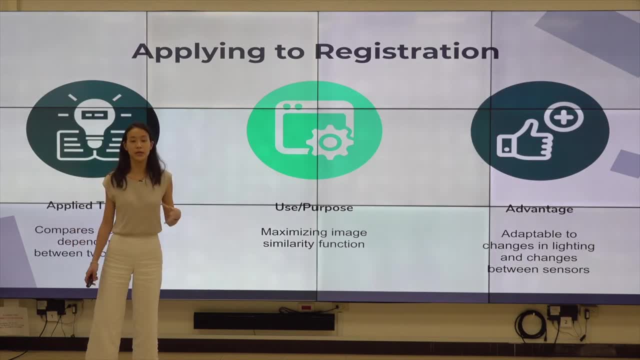 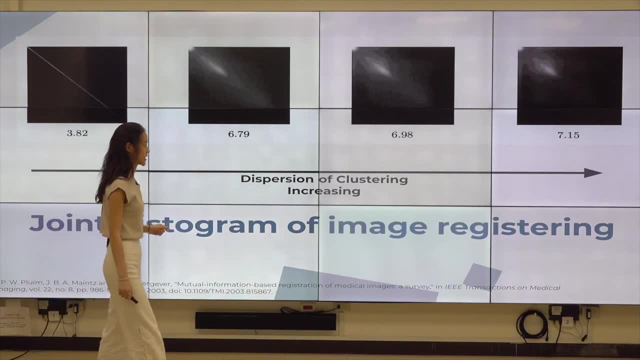 So it doesn't. it's not dependent on, for example, the machine or the MRI machine. So, talking about the joint histogram of image registering, So I'd like you guys to take a look at these four images on top. So which one? a question for you guys right now is: 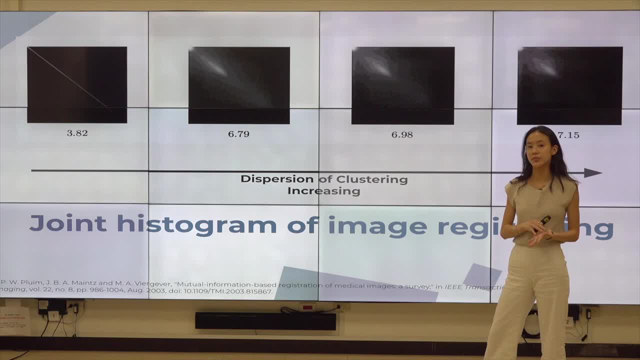 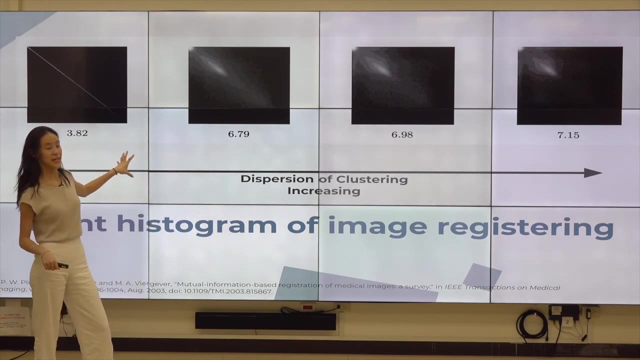 which image do you think would represent two images being perfectly registered? Do you think it's the most, the leftmost or the rightmost? So yeah, I would agree if you guys got this answer. This image actually has the most registered components to it. 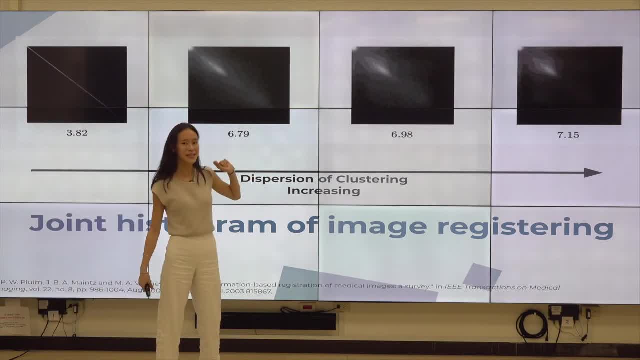 And you can see here this is the dispersion of clusters And you can see the cluster increasing. So what we see is that there is more and more clusters or more and more gray areas that we see outside of that line, which actually ultimately represents the two images. 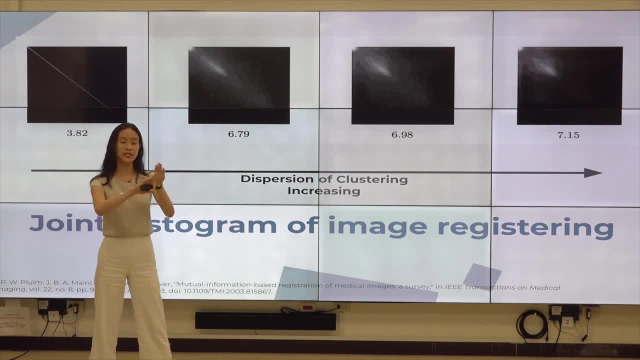 being further and further apart. So there's more differences between these two images that are on top of each other. So we see that dispersion of clustering that exists here, Whereas in this lined situation we can see the two colors as the blue and the yellow adding up together. 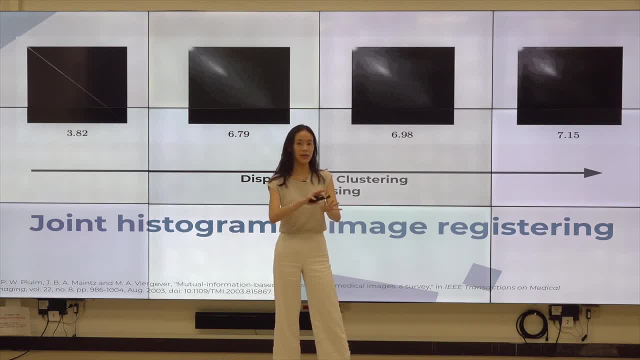 So in this situation, you would still see a little bit of the blue and a little bit of the yellow on the sides if we have the two circles coming together. However, in this line situation, you can see that that blue and yellow circle completely on top of each other, creating that green color. 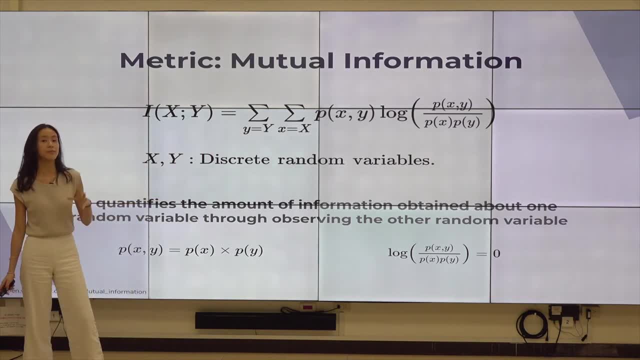 So, going on to talk about the mutual information, so the mathematics behind it, this is basically what we see. So this is a very more or less complicated kind of concept or mathematical idea, and one thing that I'd like to note, or two things that I'd like to. 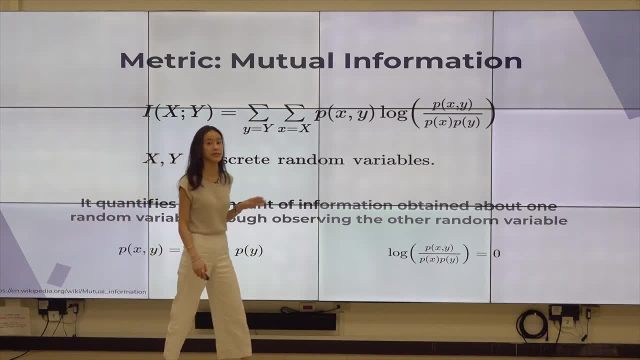 note is the fact that x and y actually represent the discrete, random variables that we talked about. so the blue and the green or the blue and the yellow would represent the x and y in this case, and what mutual information does is that it quantifies the amount of information obtained. 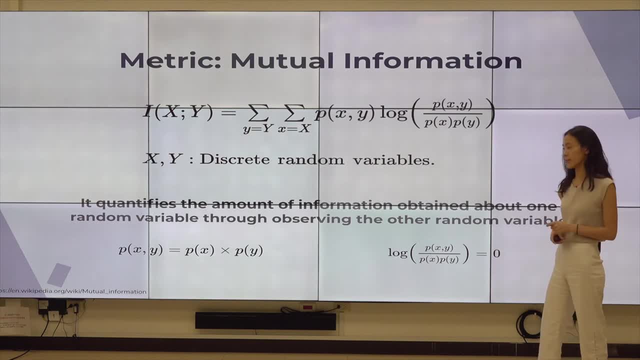 about the random variable through observing the other random variable. So one thing that I'd like you guys to remember is you, we know that if these two random variables are independent, then we would know that the log of this would actually equal to zero. so that's something to keep. 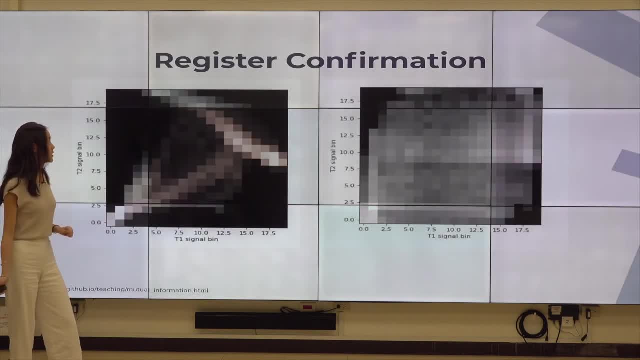 in mind of So going back and emphasizing the whole idea of image registration and mutual information, again to confirm that our images have been registered. a lot of times we would look at these pixelated images, So do you think the left side or the right side has been more or less? 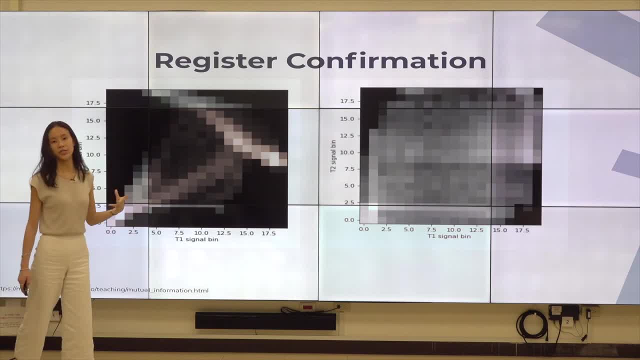 registered. So which one do you think has a higher registration or a better registration output? so yeah, I would agree with you. this image is a lot clearer in terms of the colors that we see in the clarity, whereas this one has a lot more gray scale to it. so you see, these different kinds. 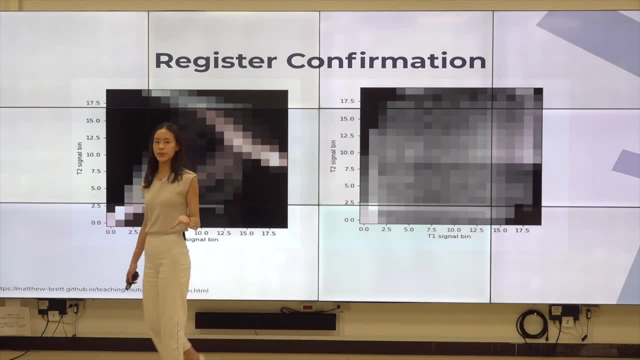 of grays and whites and blacks in there, which shows that the image was not as well registered as this image, which is very, very clear in terms of clarity and where, for example, objects are. So if this were an apple, let's just imagine these two images both being apples. what you would see in this case is: 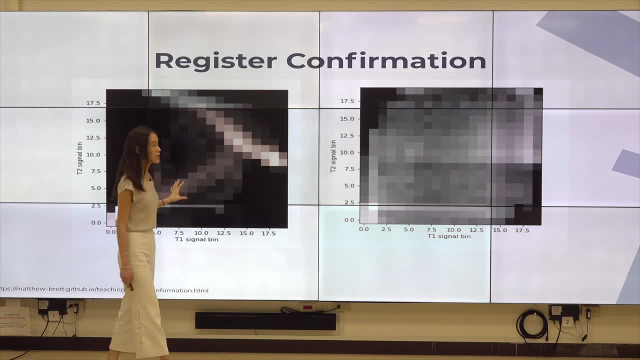 a massive red area in that middle to represent the shape of the apple that you'd be able to recognize, whereas in this situation you may have a little bit of pink on the outside and on both sides of that apple shape for you to not actually be able to distinctly recognize it as a as a shape of an. 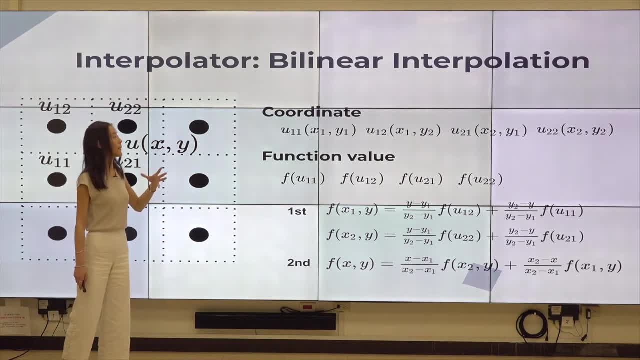 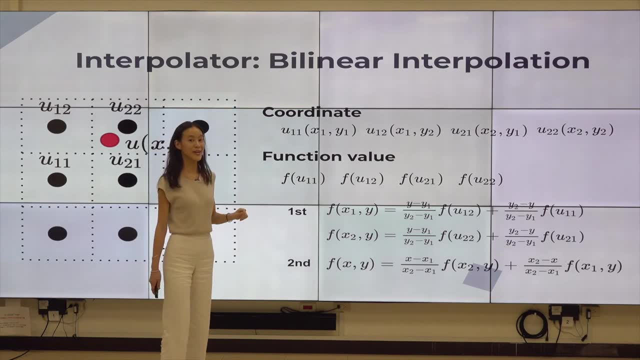 apple. And so, talking about the interpolator which is, in our case, we use by linear interpolation, so this is the mathematics behind bilinear interpolation. it's very simple in terms of how you just set the coordinates, or you, you have these coordinates that you have, you put it. 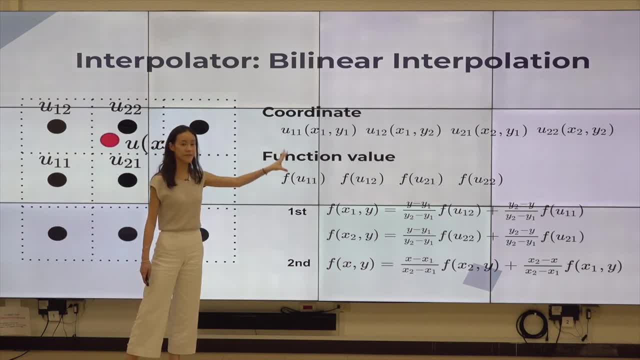 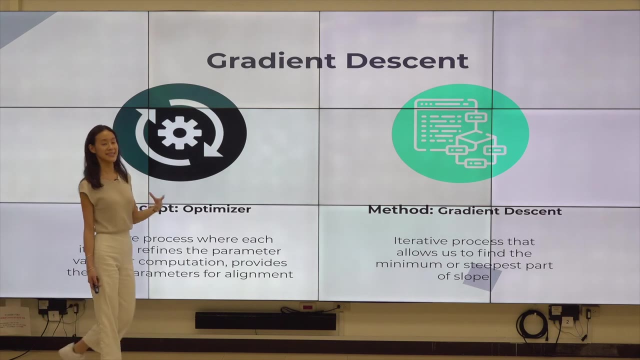 into these function values. so you have multiple functions that are defined by each of these points, in order for you to be able to determine where that exact point is relative to the other points that exist using these equations. So, going on to talking about gradient descent, as we talked about, 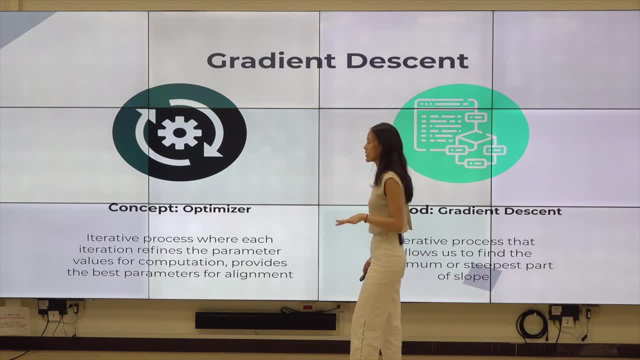 before gradient descent is. the concept is that it is an optimizer and so it's an iterative process where each iteration actually refines the parameter values for the computation so that it provides a best parameter for alignment and in the case of classification, as we saw before, it is that back. 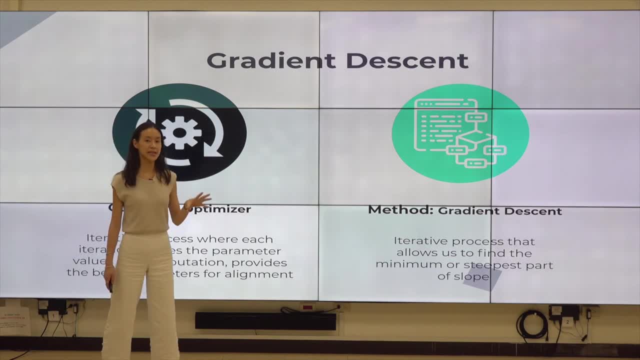 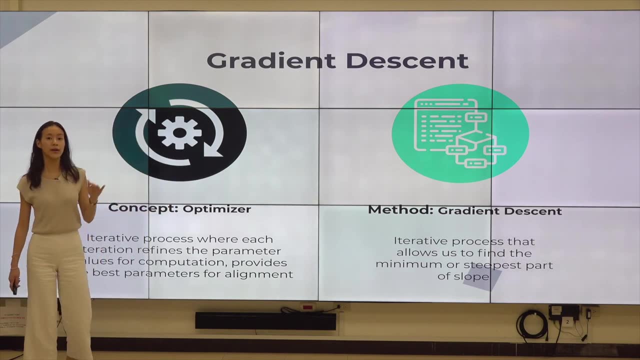 propagation method. where it is, it uses gradient descent in order to find the most accurate gradient descent to represent each of these nodes. In this case, it is going through that iterative process to find the parameters that allows us to be able to achieve the best alignment between two. 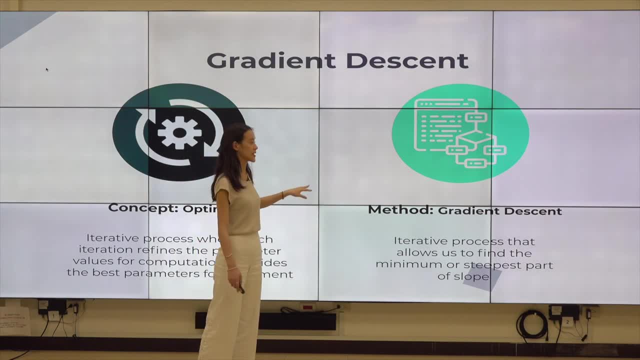 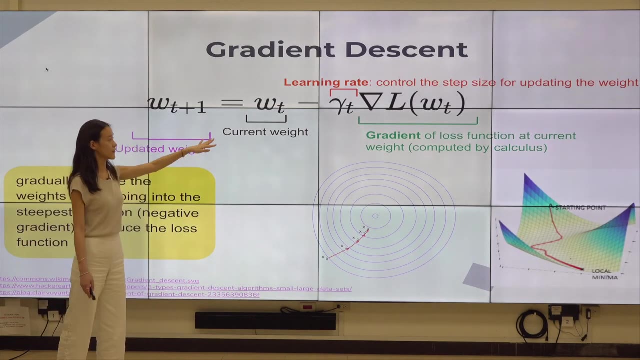 images, and so, in this case, for our optimizer, as I stated before, we're using gradient descent, and it is an iterative process that allows us to find the minimum or the steepest part of the slope, as we'll see in the next slide. So gradient descent mathematically refers to this thing, as we see here. 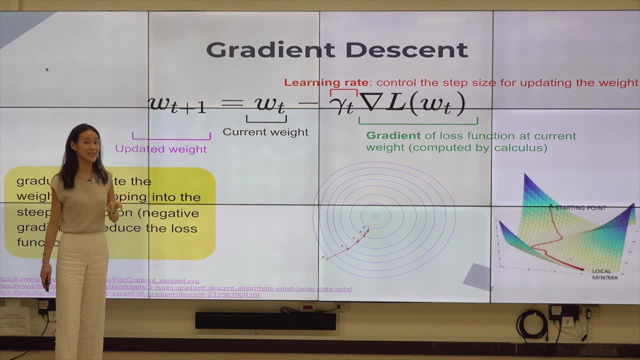 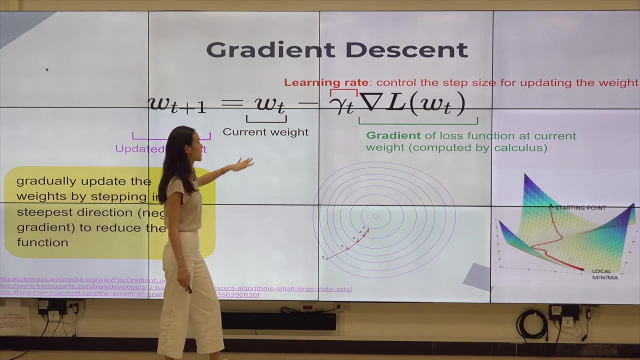 this is the updated weight. so I'm pretty sure, as you guys remember from that segmentation lecture, what we have is the constant updated weight. so this is the new origin or the new image that we talked about in the segmentation lecture, and so this is the current weight in terms of where we are. so this becomes 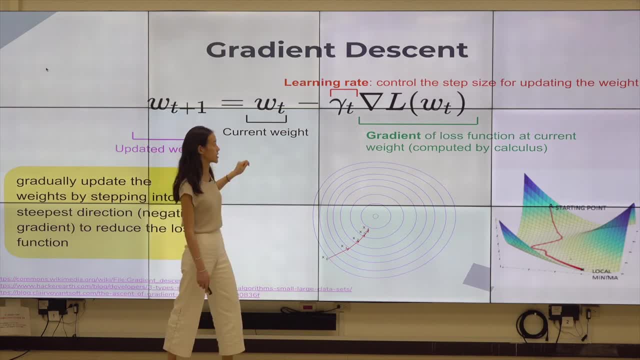 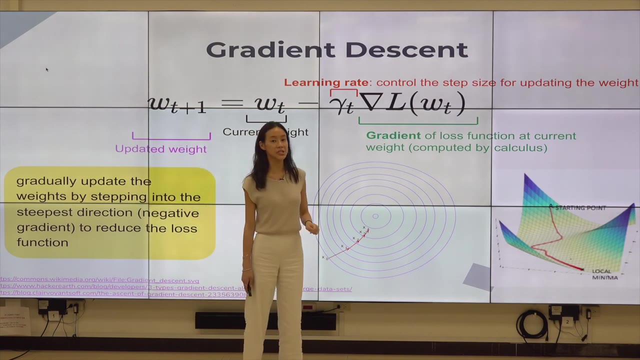 edited. every single, every single iteration and the learning rate basically defines where or how much we're learning with each iterative step and that's the gradient, or the gradient of the loss function at the current weight that we're at. so, as seen before in the segmentation lecture, I would recommend 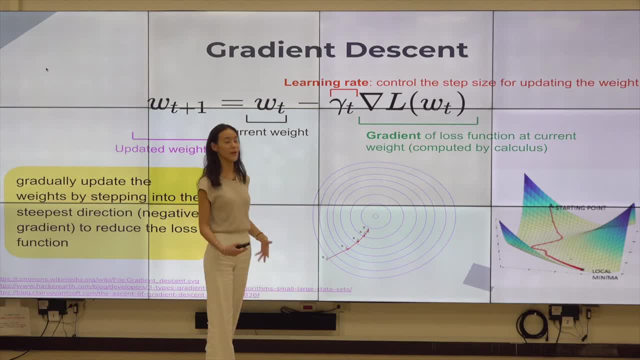 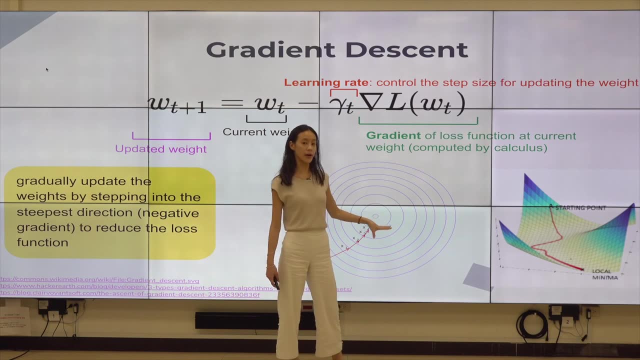 you guys to look back to it if you don't remember or if you haven't watched it. what ends up happening is that we're trying to find that steepest part in each of our functions, and so, in this case, if we're starting at point A, what? 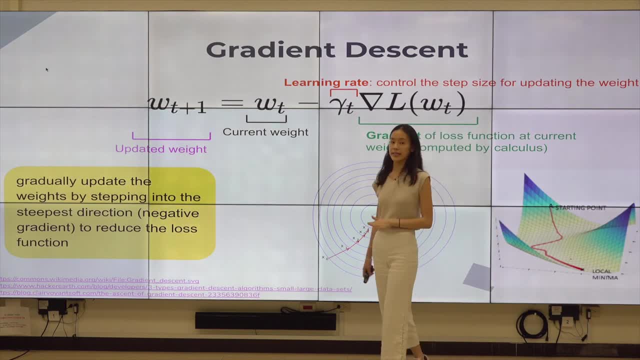 we're trying to find is that very, very minimum point through gradient descent, so through this iterative process. so one thing to note is that in the segmentation lecture we're trying to find that very, very minimum point through gradient descent, so through this iterative process. so one thing to 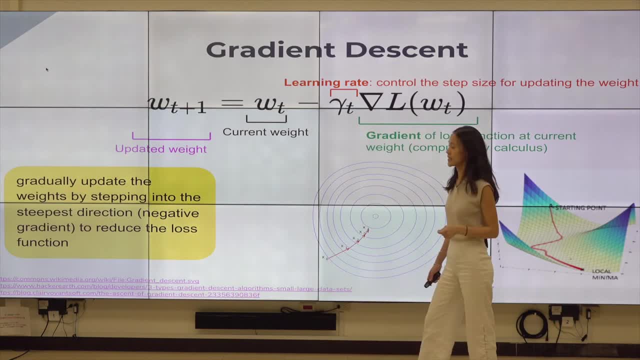 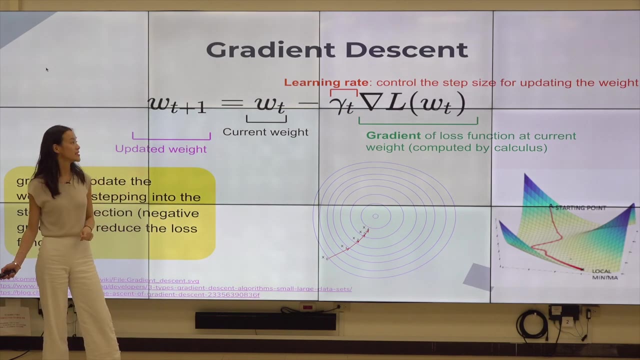 note or to remember is that it gradually updates the weight by stepping into the steepest direction to reduce the loss function. so remember it is constantly updating the weight in order to achieve minimum, always minimum. that's what I like to remember with gradient descent. so the multimodal gradient. 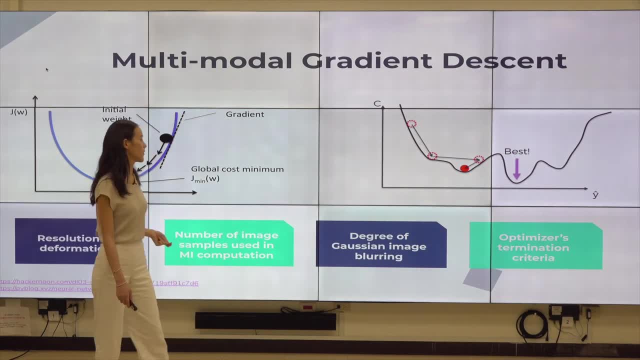 descent is actually an improvement of the gradient descent that we were talking about before, and the whole idea behind this is the fact that in a very simple function, as you see here, it is very easy for us to determine where the minimum is. it's going to be at that minimum point of the concave, of the of the concave function. 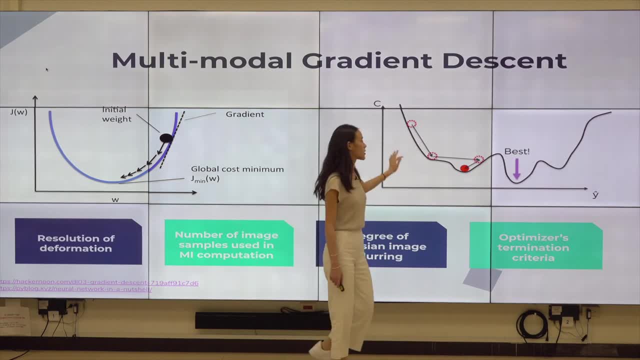 however, in a situation here where there may be multiple dips that we see, it is very easy for a function or the algorithm, through gradient descent, to define this point as the minimum. as the minimum point because a lot of times, as we stated before, what ends up happening is that, as long as there is some sort of 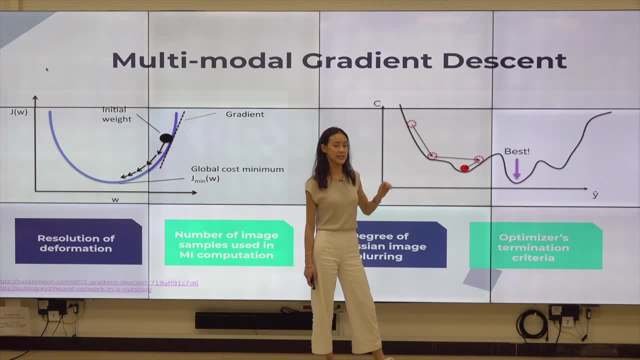 increase what the gradient descent or what the algorithm does is, it goes back, takes a step back to that very minimum point, or that last point where it was a minimum, and defines this minimum point as the very, very minimum of the entire function. However, as I stated before, in this function you see that the best minimum 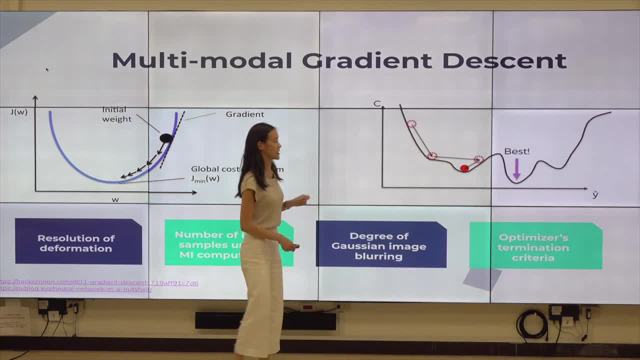 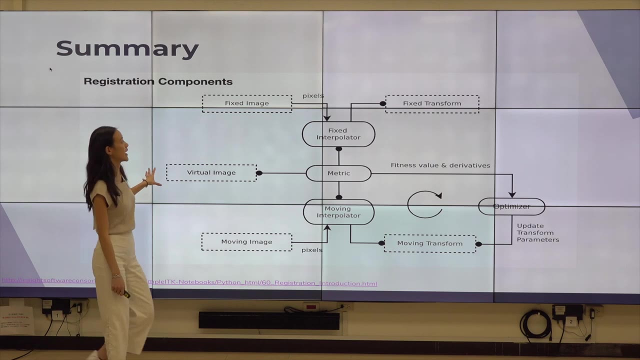 is actually here. So what multimodal gradient descent allows us to do is to be able to determine this best, this best minimum, without stopping at a local minimum. So, as a summary of the entire registration process, what I'd like to see is that what we would have that go through the workflow is we would have 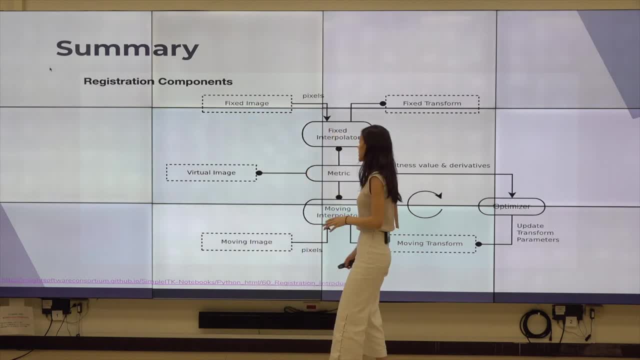 the fixed image and the moving image. that basically goes through and we have that metric- and it goes through that training process of continuously registering. so think of your arms in the same way, where you go through that iterative process to be able to find the optimal transformation function for us.